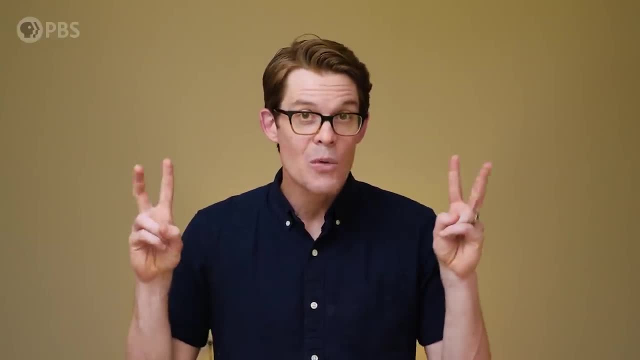 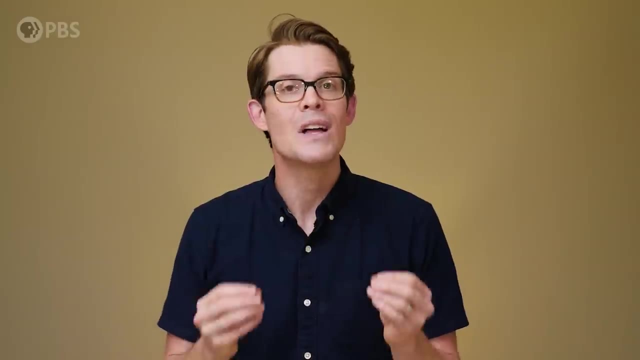 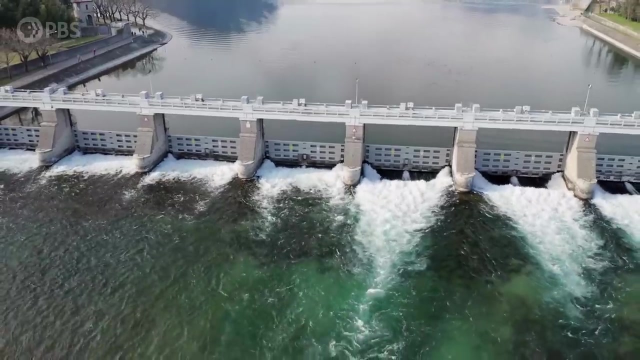 But in the context of environmental science, when we say generating energy, we're talking about the conversion of various types of existing energy out in the world into electrical energy that we can move and actually use, And most of the time in power plants, from coal to gas to hydro, we create this electron. 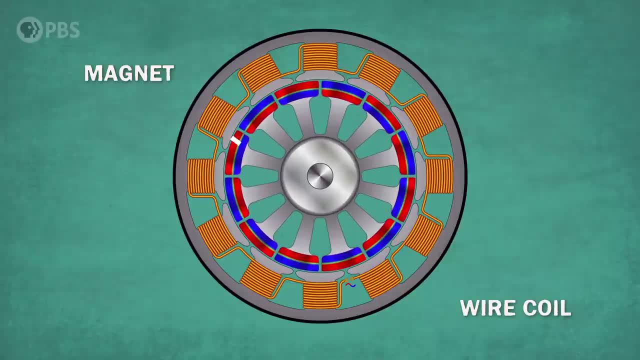 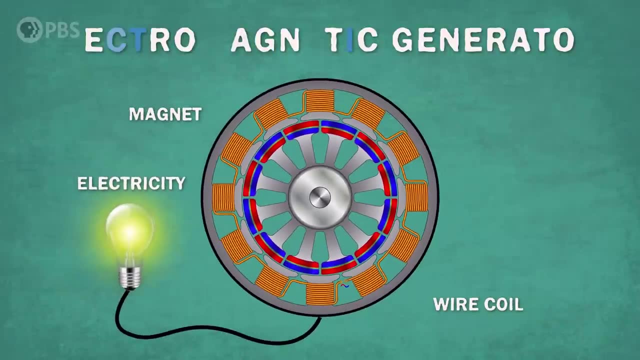 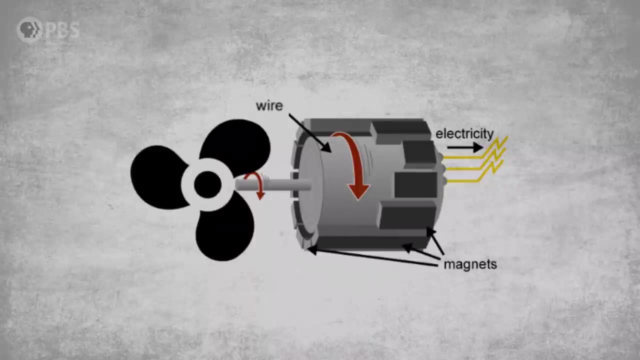 parade by rotating coils of wire around really big magnets. The magnetic field moves the electrons, And the electrons within the wire generate electrical energy. This device is called an electromagnetic generator and it transforms mechanical energy into electrical energy. to keep the generator spinning, we use a turbine. 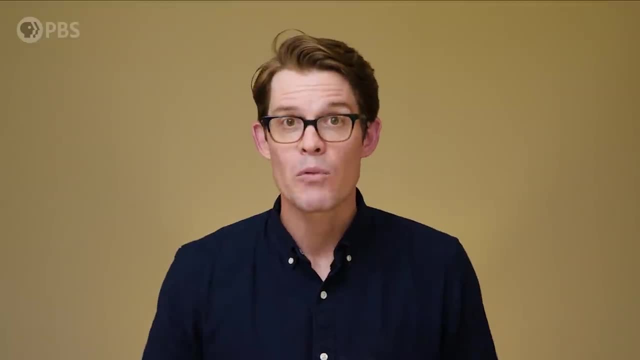 It's basically a big fancy looking fan thing And that is kept rotating by our energy source, which could be flowing water or wind, but is often steam coming off of a heated liquid. This chart summarizes the primary ways in which we generate electrical energy. 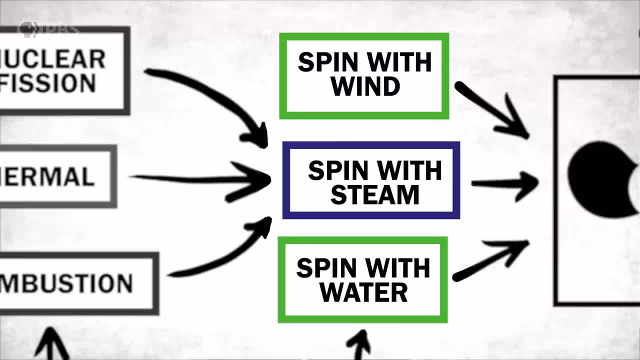 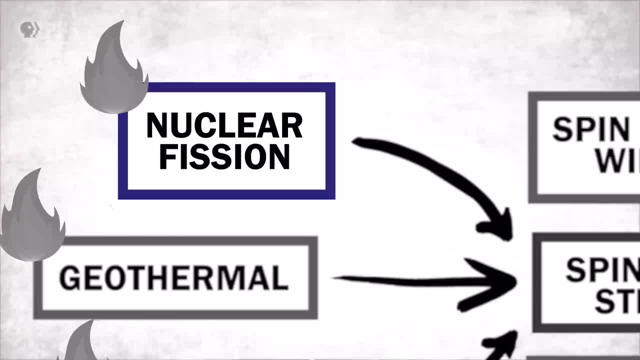 We've got burning fossil fuels, We're capturing wind and flowing water Or tapping into the intense heat under the ground. Even splitting atoms, like in a nuclear power plant, ultimately generates energy. in the same way, Uranium atoms are split to generate enough heat to boil water, to make steam, to spin a. 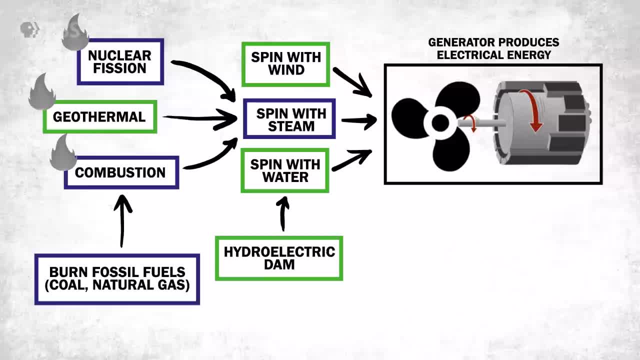 turbine to rotate the generator to make energy. Of course, often the corner there is the primary way we generate energy without an electromagnetic generator. Solar Photovoltaics convert light energy from the sun into electrical energy without the need for bulky turbines or generators. 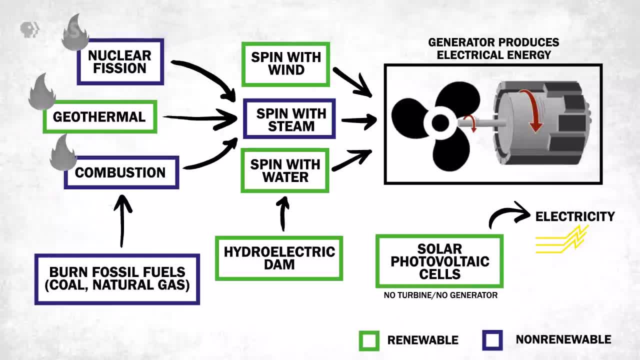 This chart also highlights which sources are renewable, meaning we can never run out, no matter how much energy we make from those sources. And the little flame emoji? Well, that means those sources generate electrical energy and can be used for heating. It's a term called cogeneration. 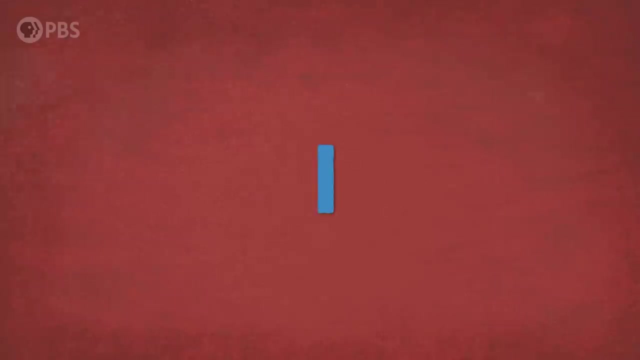 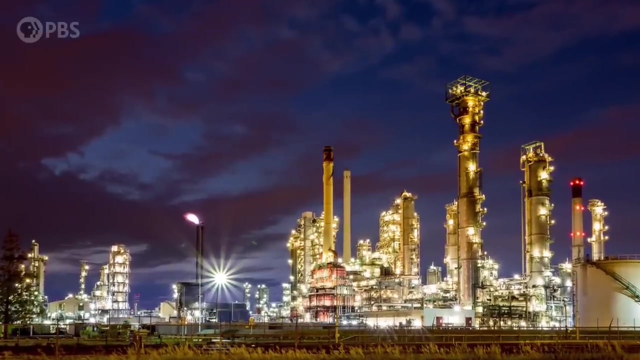 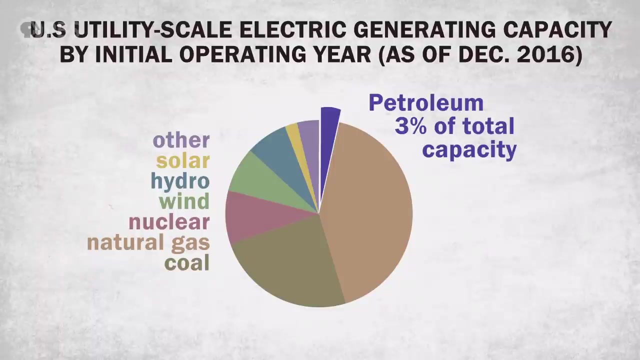 And there's one major fossil fuel missing from this chart: Oil. Crude petroleum isn't really used to create electrical energy anymore. While oil-fired power plants do exist in the US, they only make up 3% of energy generation, But oil is still a major form of energy and carbon emissions just mainly in transportation. 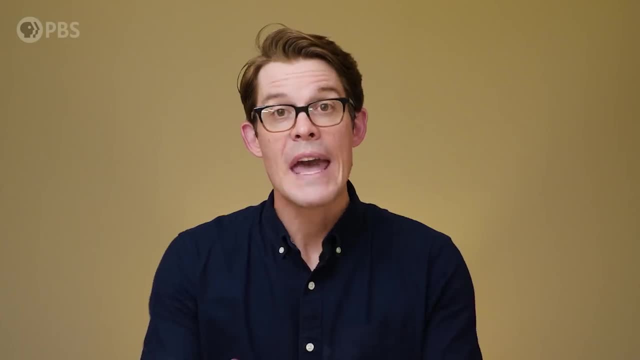 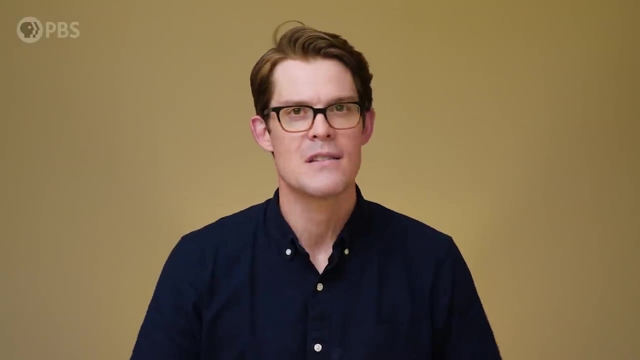 and in making plastics, which we will talk about shortly. Okay, so we have all these ways of generating energy. Why does an environmental scientist or just the average person need to know about all these? Well, as we talked about in the climate and air episodes, each of these forms of power. 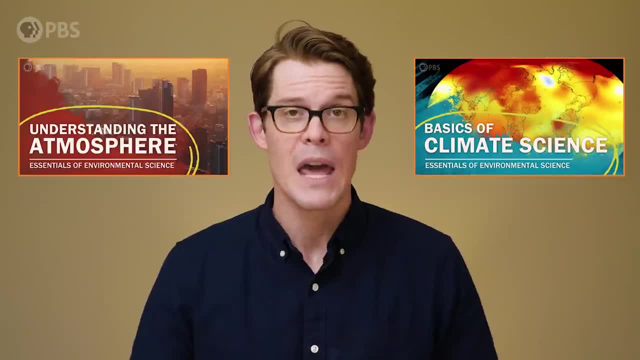 generation carry their own risks for making a big mess of the planet, and some far, far more than others. So for each of these energy sources, we need to know how it works and why, And that's what we're going to talk about today. 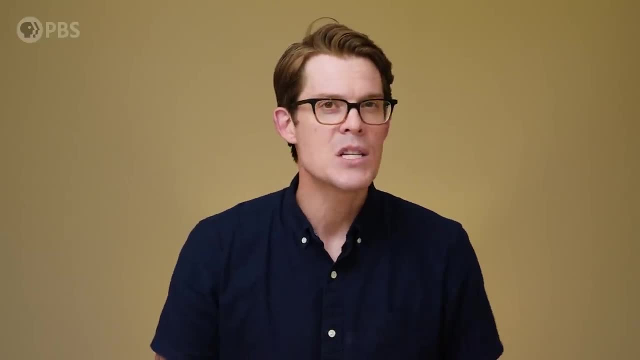 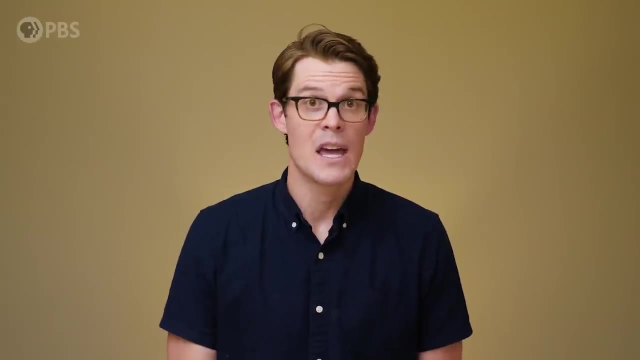 So let's get started. What are the pros and cons? Knowing more about each of these can help us transition to a more sustainable energy production in the future Or now. Let's start with the most common way of generating energy today: burning fossil fuels mainly. coal or gas. Now, when these combust, they release huge amounts of energy. But where does all that energy come from? What even are fossil fuels? Well, like many things on the planet, it all starts with the sun. Millions of years ago, plants loved sunlight, just like they do today. 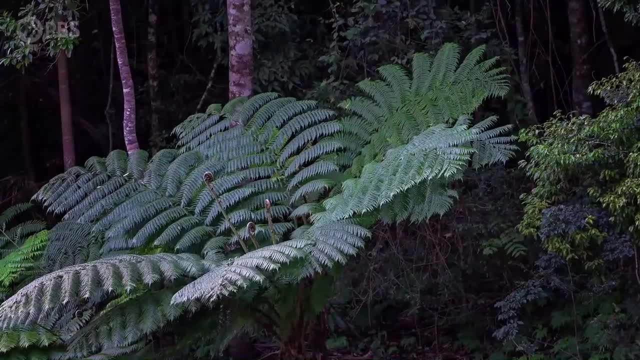 All plants, from marine phytoplankton to savannah grass, all started with the sun, And that's why we're here today. So here's the first one. When plants were growing, they needed to be fed with the sun. When plants were growing, they needed to be fed with the sun. 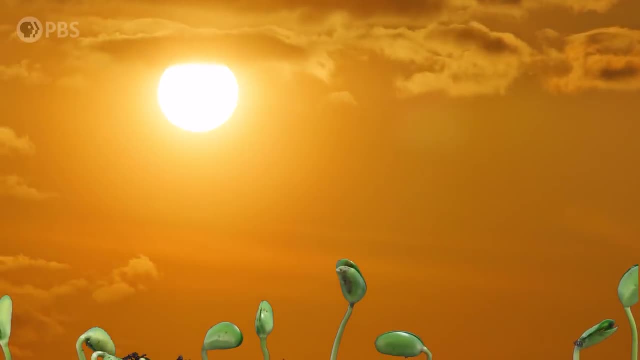 The sun is also a source of energy. It rose from the sun to the earth When plants were growing. they needed to be fed with the sun. All of this energy, from the radiated grasses to those massive fern palm things that flourished. 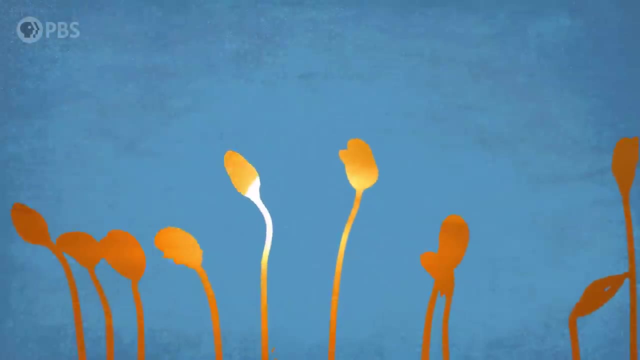 during the Carboniferous Period rely on sunlight for photosynthesis, And through photosynthesis that light energy from the sun is stored in the plants' bodies. Generally we can track that energy as it moves through the food web from producer to consumer or to a decomposer. 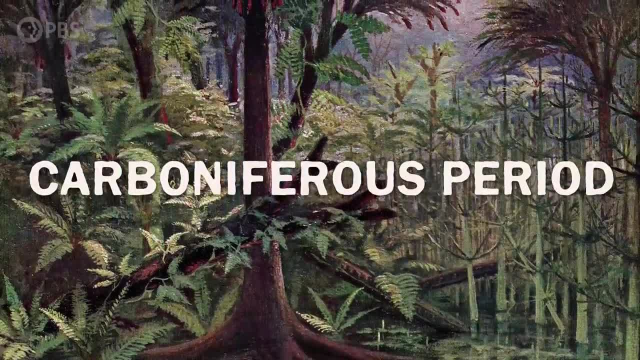 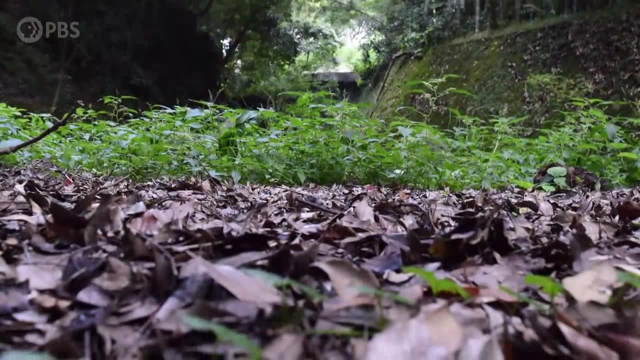 But during the Carboniferous Period, when most of our fossil fuels were created, there was such an abundance of plant life that when those plants died, not all of them were eaten or decomposed. Instead, those plants and all of their stored energy from the sun got buried under layer. 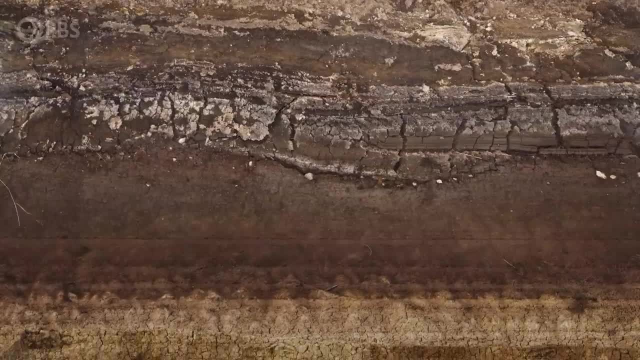 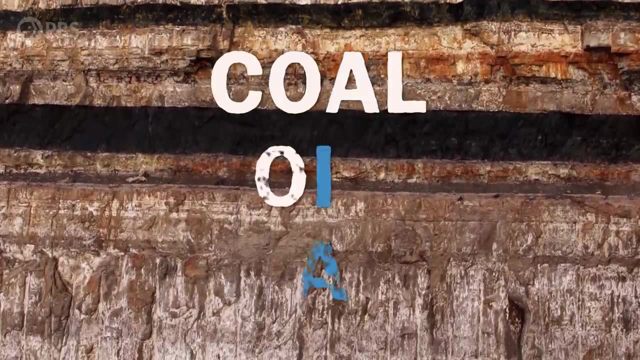 after layer of sediment, After millions of years of heat and pressure. from the weight of all that earth, the organic materials in those plants became the hydrocarbon fossil fuels that we use today: coal, oil and gas. The difference in the formation of those three is mostly a matter of how much heat and pressure. 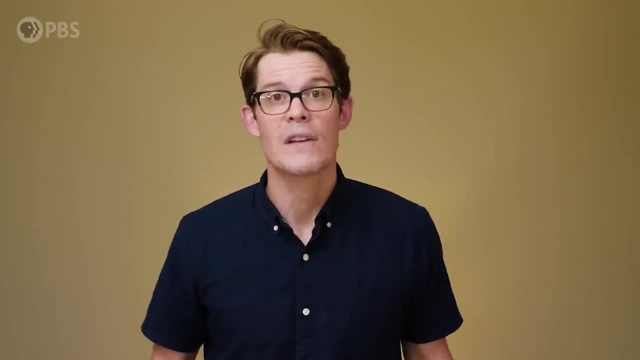 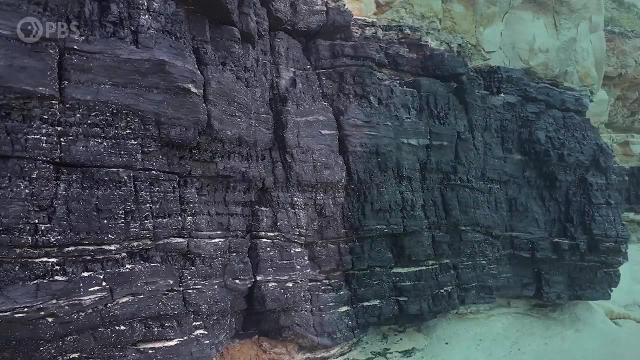 they were exposed to during formation. And once people figured out there was eons worth of stored energy underground, they developed special mining techniques to get it out. So for coal, if the coal seam or layer of coal isn't too deep underground a technique, 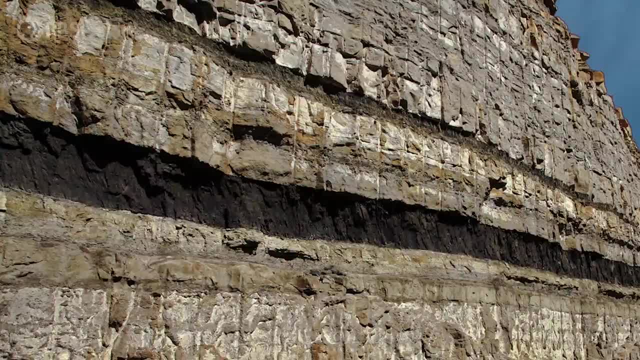 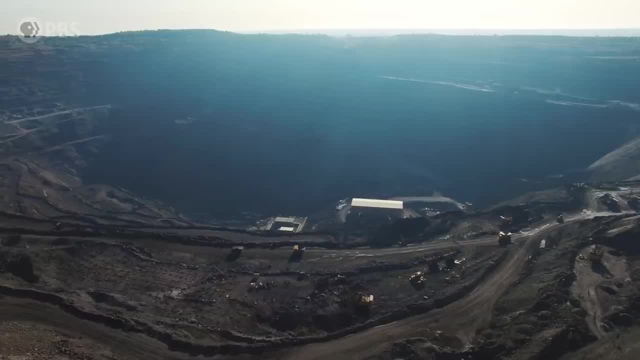 called surface mining, will be used. The soil and rock above the coal, called, unironically, the overburden, gets removed by massive surface miners and dump trucks, either by burrowing down into the ground or grinding away the surface layer which, as you can imagine, isn't that great for whatever. 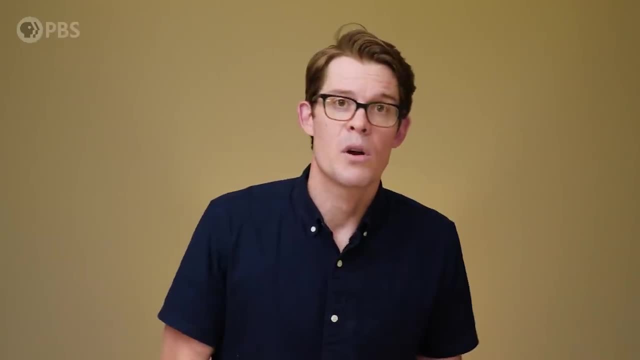 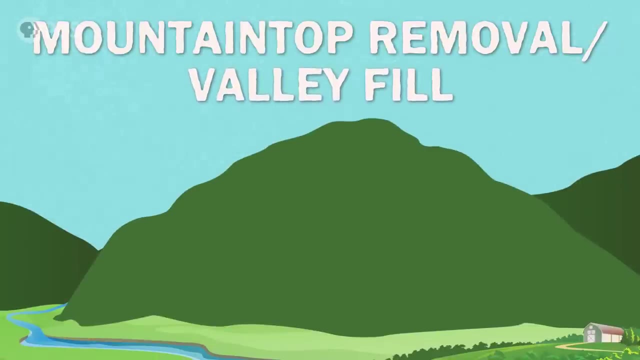 ecosystem was there before And wherever we dump, all that overburden also has serious impacts on the ecosystem. Another form of surface mining is called mountaintop removal- valley fill. If there's a suspected coal seam inside of a mountain, they'll literally blow up the 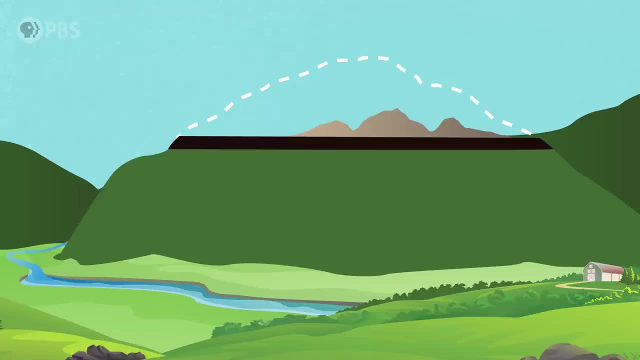 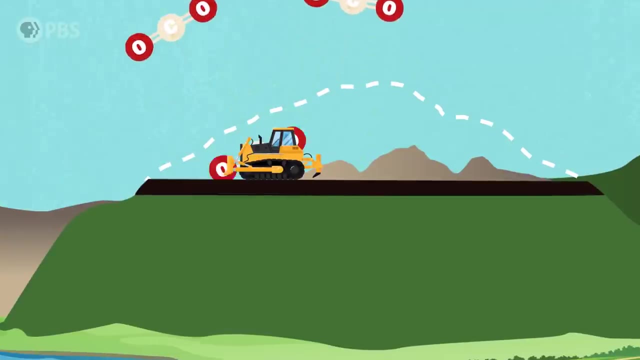 mountaintop or ridge in order to start a surface mine and then dump the overburden in a nearby valley. If that wasn't bad enough, the process of surface mining also releases large amounts of carbon dioxide, which, as you know from the last episode, is a powerful greenhouse. 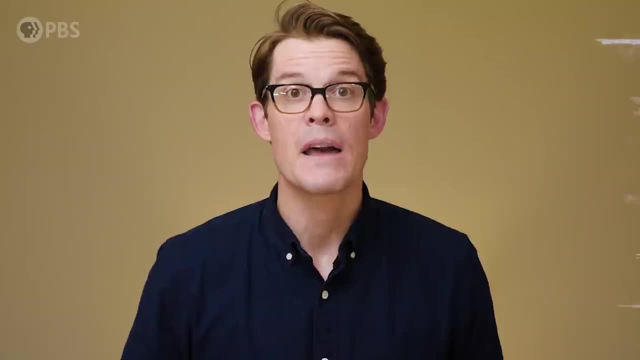 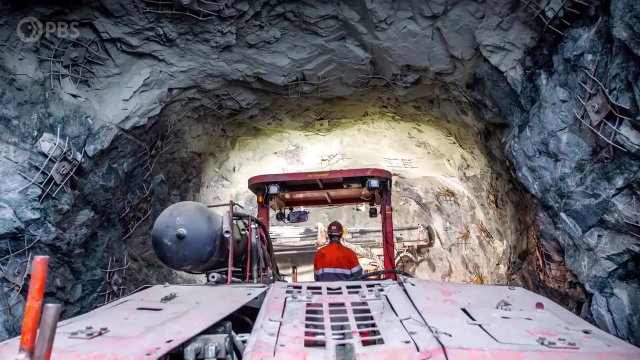 gas involved in climate change. To get at the really buried stuff, miners turn to subsurface mining. In this method, large shafts and tunnels are dug into the ground. Humans and large machines travel down those tunnels to extract the coal. This type of mining is more expensive and the process is more dangerous to humans than 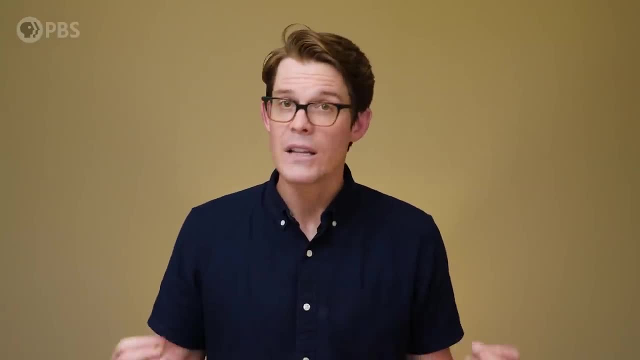 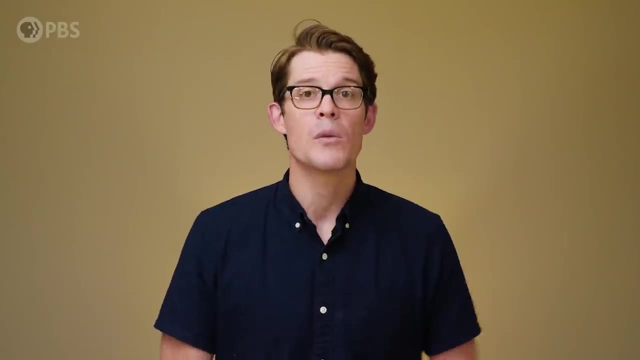 surface mining. Surface and subsurface mining can radically alter the topography of the earth, resulting in higher rates of erosion as well as habitat loss, and can cause severe water pollution issues. As water flows through these mines, it runs across coal waste, picking up sulfur and creating 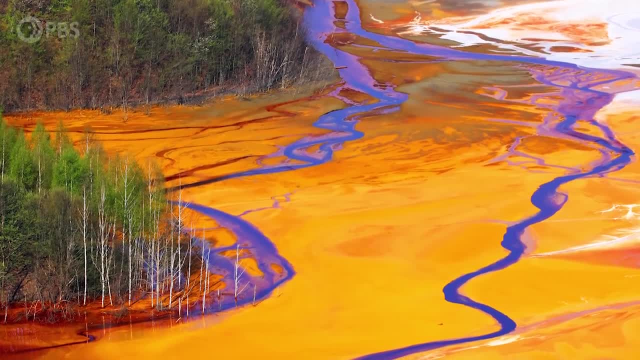 sulfuric acid. This acidic water leaches out metals which can be toxic. One of the most common sources of sulfuric acid in the world is coal. It's the most common source of sulfuric acid in the world. Once mined, the coal is transported, often by train, to coal-fired power plants. 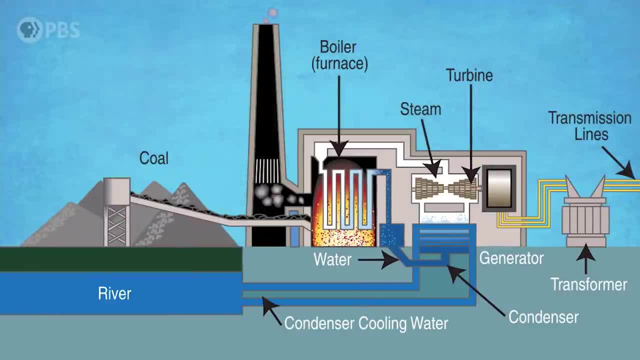 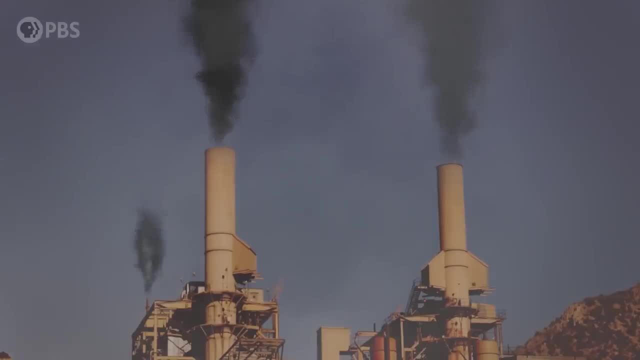 At these facilities the coal is burned and the heat generated is used to boil water, to make steam, to turn the turbine and to spin the generator to produce electrical energy. But as the coal burns it releases pollutants into the air that harm both the environment. 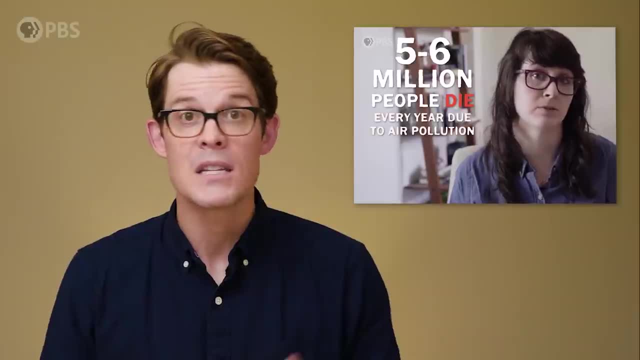 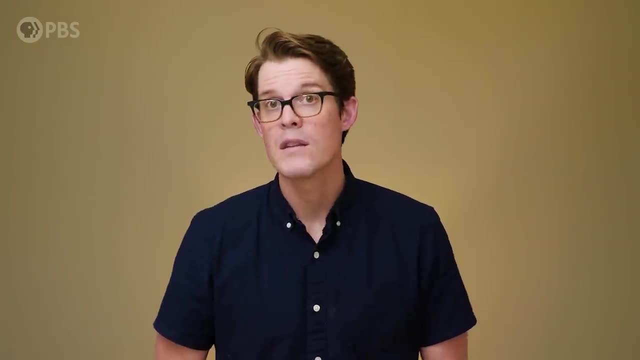 and human health. In the air episode, we talked a great deal about the different types of pollutants emitted during this combustion process, and none of them were good for us, Which is part of why the number of coal plants, especially in the United States, is so high. 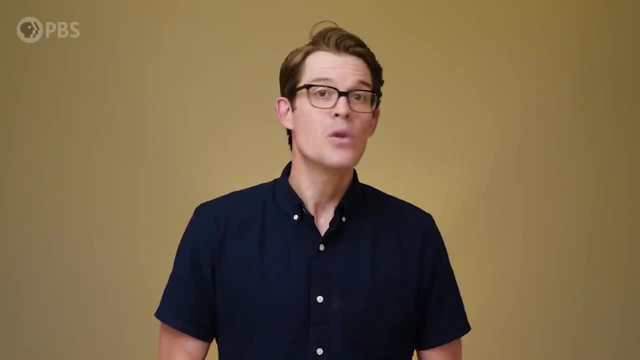 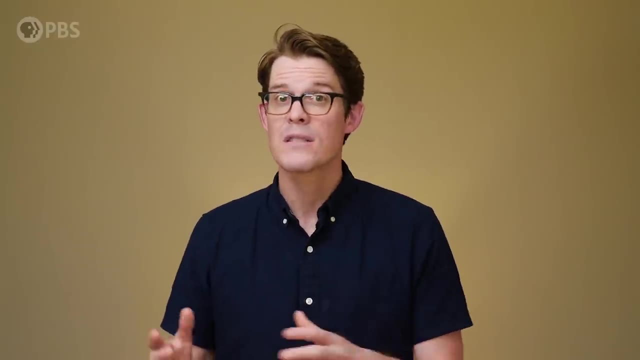 The number of coal plants in the United States is. the number of coal plants in the United States is going down. Not only do they produce massive amounts of carbon dioxide emissions and air pollutants, but these days, coal mining and coal-fired power plants have a hard time competing economically. with other, cheaper forms of energy production. Oh, and one last thing about coal. When coal is burned for energy, we're left with all these extra particles and residue called coal ash. To keep the coal ash from getting into the atmosphere, coal-fired power plants often 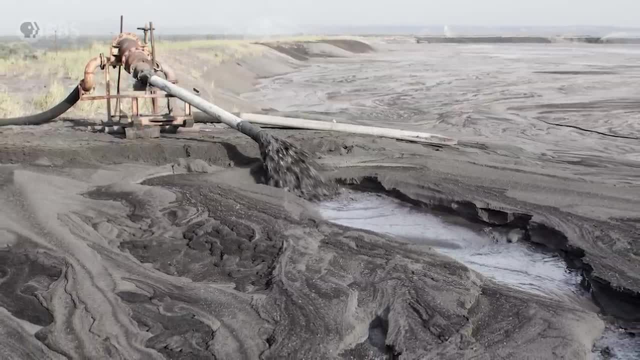 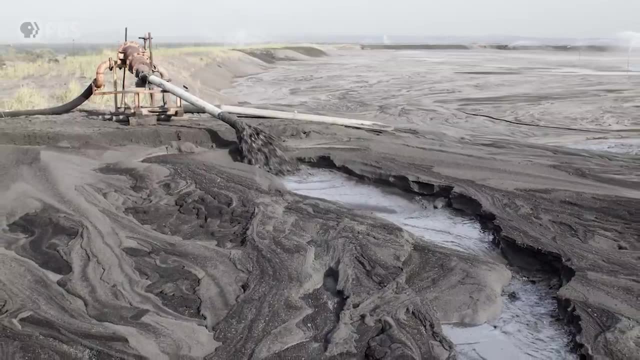 have these kind of landfill ponds where the ash gets dumped, but a large hazard like a flash flood or a dam or a fire is not enough to keep the coal ash from getting into the atmosphere. A dam bursting can easily flood those ponds, releasing toxic coal ash sludge everywhere. 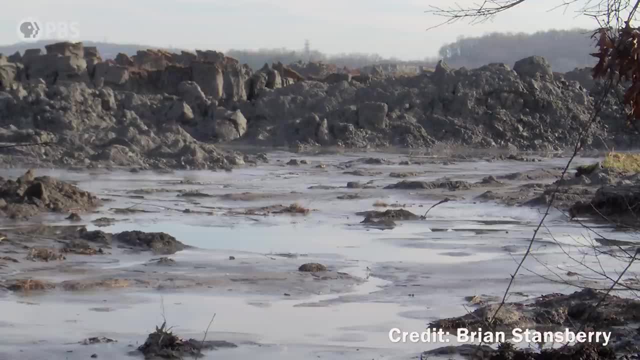 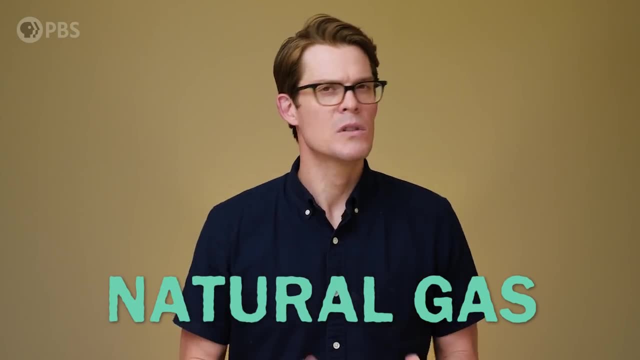 This happened in 2008 in Tennessee, when billions of gallons of coal ash slurry were flooded onto the surrounding areas. Next, gas, or what many people call natural gas, but should really be called fossil gas, because there's a whole history about people calling things supposedly natural, which we 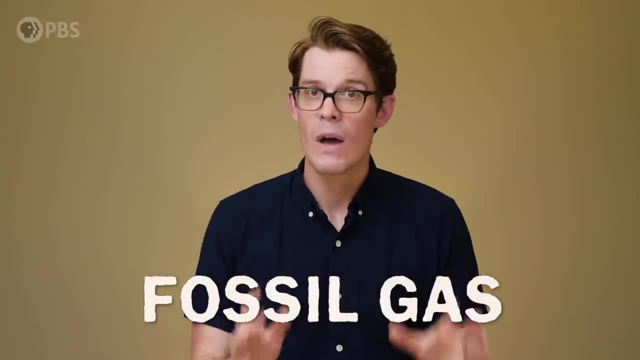 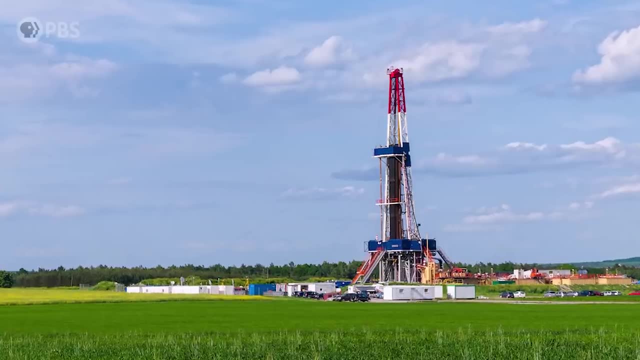 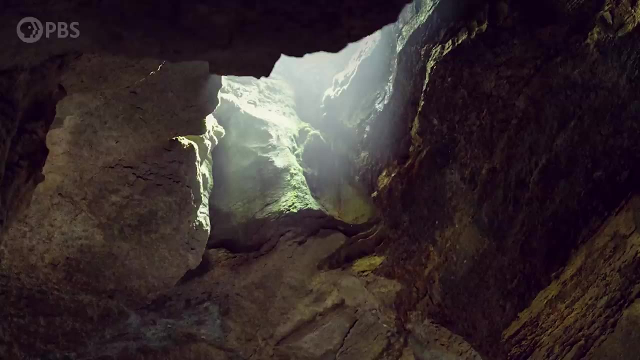 can talk about another time. Like coal, gas comes out of the ground ready to use, but gas releases less air pollution than coal when burned. Extraction and use still cause a lot of environmental problems. Gas is mainly methane, and a lot of it is located in pockets that are sandwiched between 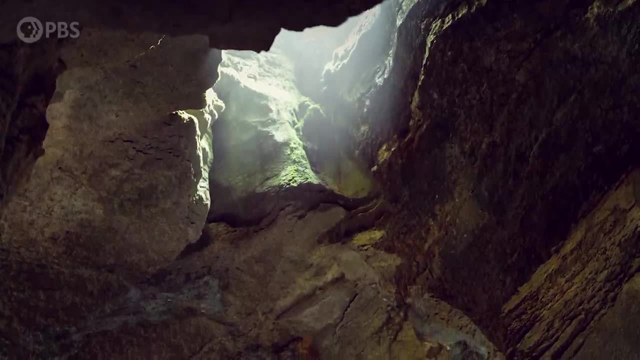 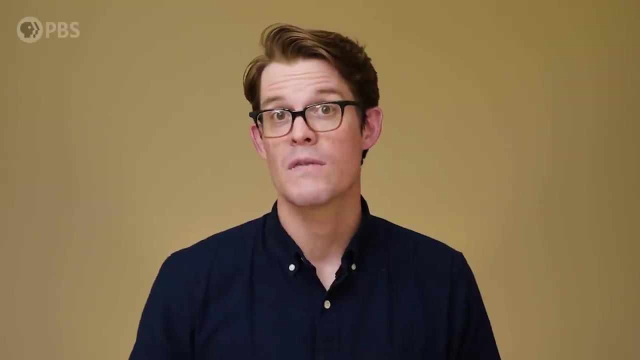 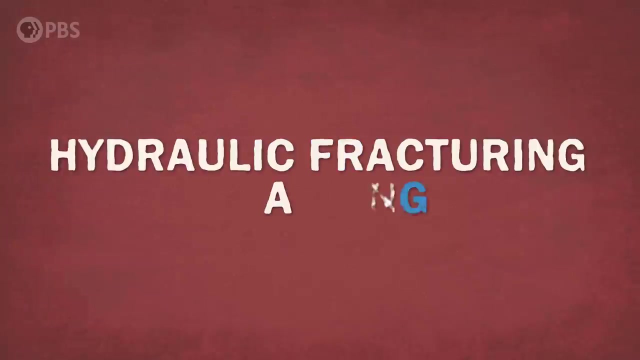 layers of rock. This is relatively easy to drill down and extract- Way easier by comparison to building a massive surface mine that relies on heavy machinery. But there are also massive stores of gas located in the pores of underground rock formations. To extract this gas, a process called hydraulic fracturing or fracking was developed. 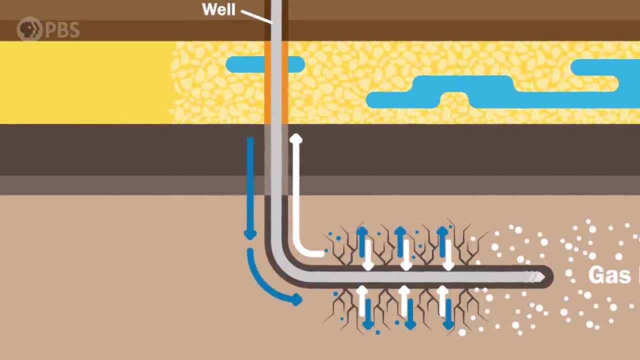 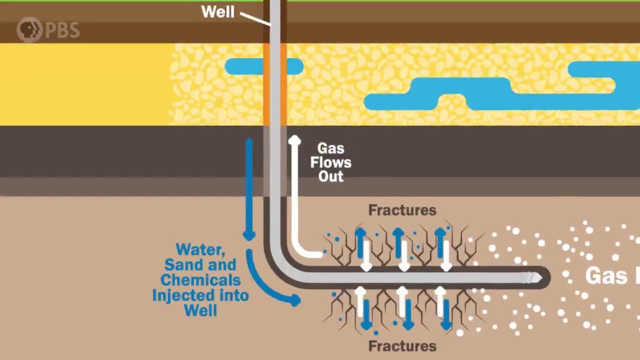 In fracking, holes are drilled. These holes are drilled deep underground into these rock formations and a mix of pressurized water and sand and chemicals is then injected into the hole to crack open the rock and release the trapped gas. Fracking opened up access to a lot of gas that had previously been too difficult or 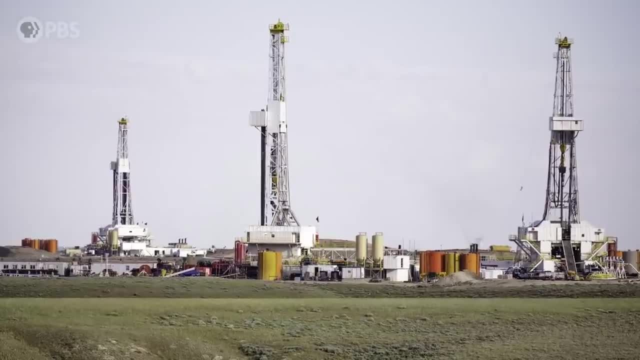 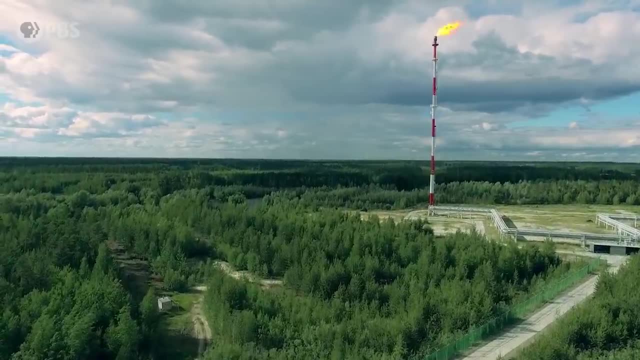 expensive to extract, making gas a much more common and cost-competitive energy source for generating energy in the last few decades. While burning gas releases less air pollution and greenhouse gases than coal, when it's burned, it's still a big source of emissions. 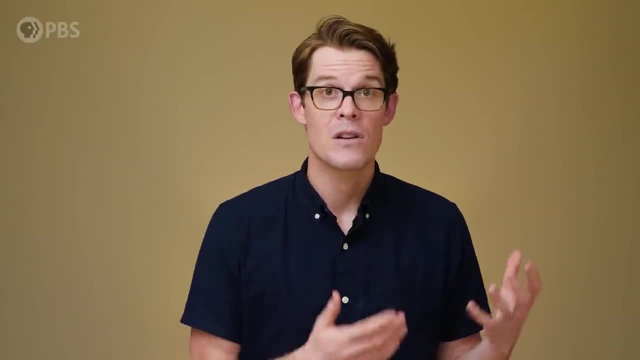 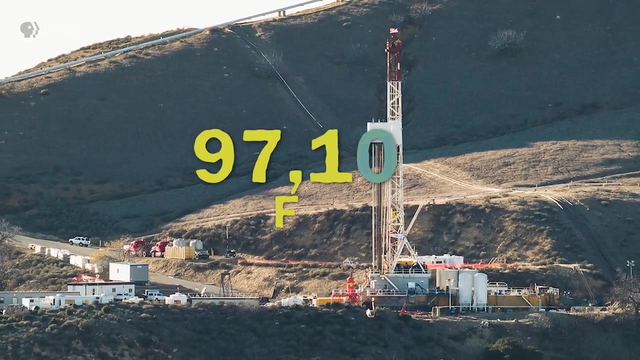 And not only that: the fracking process can accidentally leak methane either directly into the atmosphere or into the groundwater below. In 2015,, a gas well in Aliso Canyon leaked an estimated 97,100 tons of methane into the atmosphere. And once methane's there, it's a very powerful greenhouse gas and a major contributor. 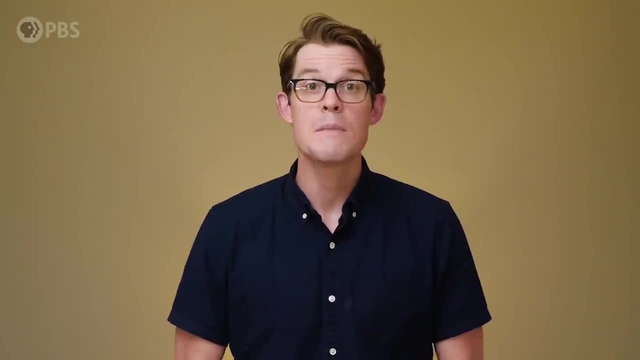 to climate change on its own. When methane or fracking liquids seep into the groundwater below, it can be dangerous to living organisms, including humans, who may use that groundwater as a drinking source. Okay, I've had enough of combustion, Let's get back to work. 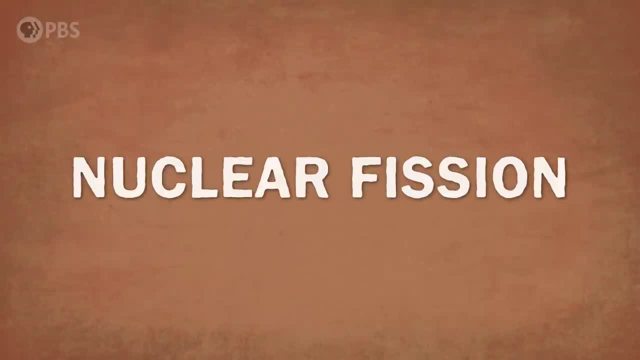 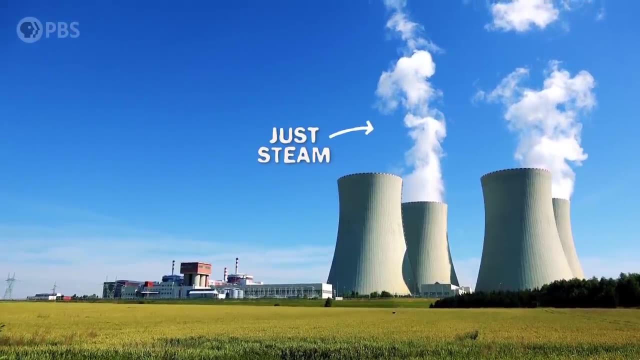 Let's talk about other forms of energy generation, like nuclear fission. Fission releases energy by the splitting of atoms, not combustion. So one powerful benefit of nuclear energy is that it does not release air pollutants or greenhouse gases as it generates energy. 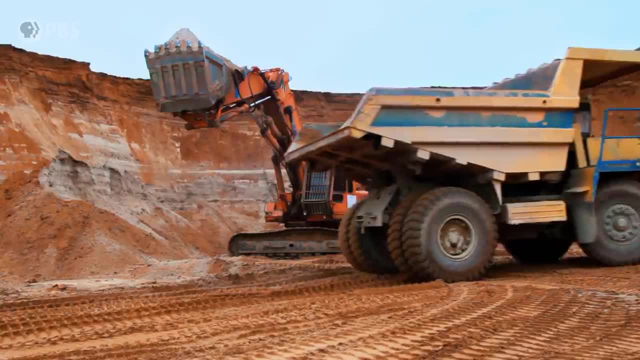 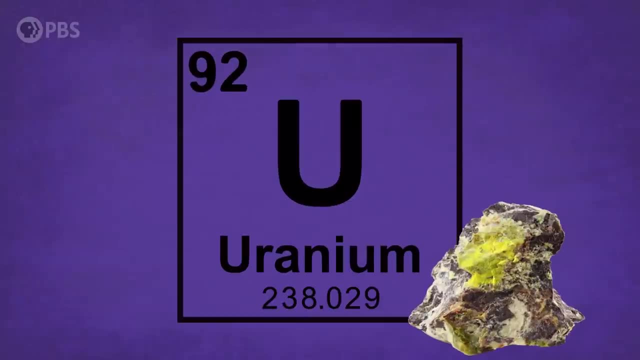 Fossil fuels are burned during the construction of the power plant and during the mining and transportation of nuclear fuel, but once a reactor's up and running, there's basically no emissions. The fuel for a nuclear power plant is uranium. Splitting open this radioactive nucleus by bombarding it with neutrons makes it a nuclear. 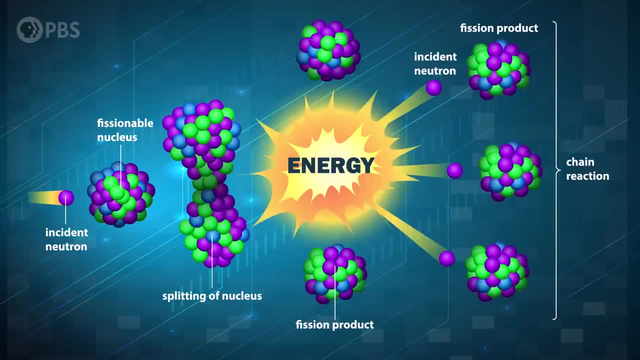 power plant, making new radioactive particles and lots and lots of energy. Once the fission chain reaction starts, it wants to keep going, so it has to be carefully monitored and controlled so that it doesn't produce too much heat. The heat from fission, like in other power plants, is used to boil water, make steam. 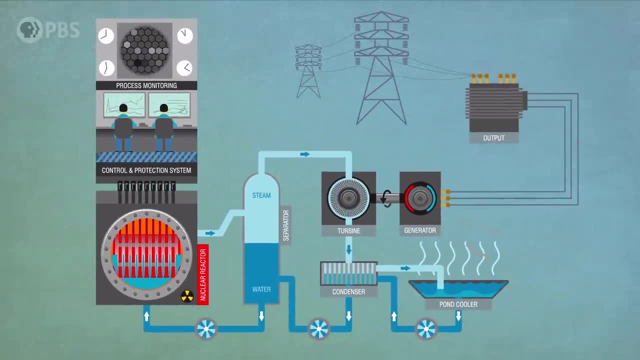 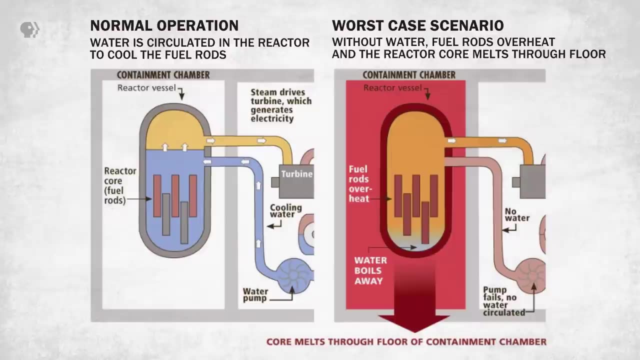 and spin a turbine to generate energy. The temperature of the nuclear reactor itself must also be controlled. If it's not regulated and constantly cooled down, then it could overheat and cause a nuclear meltdown. During a nuclear meltdown, something goes wrong with the circulating water surface. 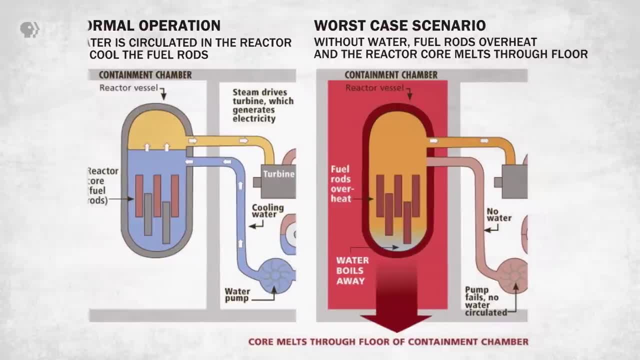 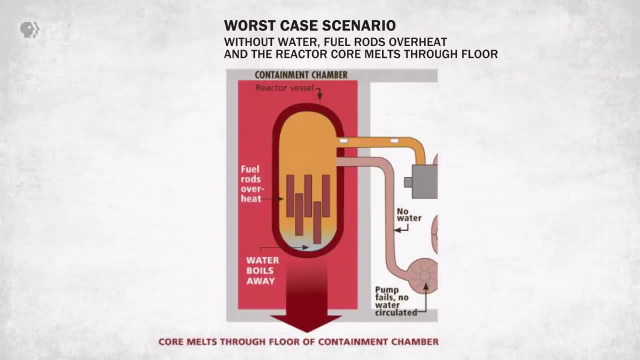 a system that's used to regulate the temperature of the reactor, and if this water circulation system fails, the nuclear reactor overheats, melting the protective containment, building itself and releasing radioactive material. The world has seen three big nuclear meltdown accidents in the past. 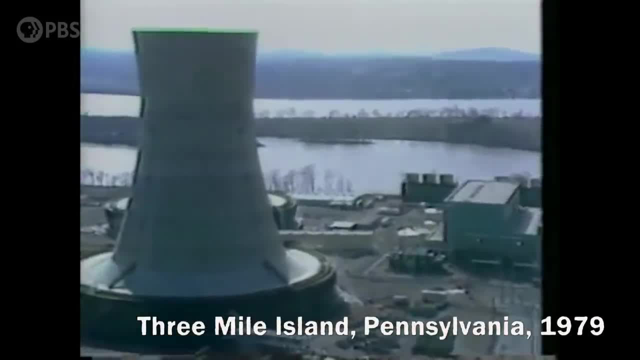 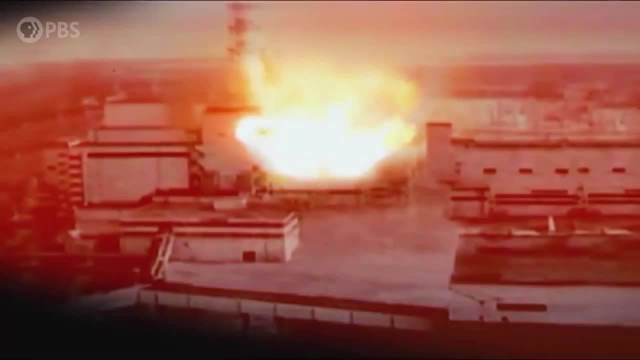 The largest US nuclear accident was a partial meltdown at Three Mile Island. It didn't result in any deaths, but it caused panic and concern about whether or not to build more nuclear power plants. Another accident was Chernobyl, where thousands of lives were lost after radiation and the 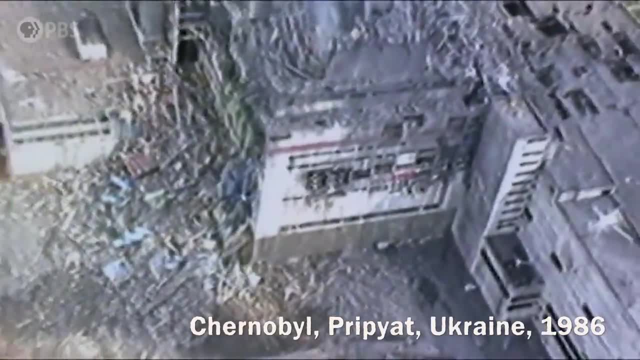 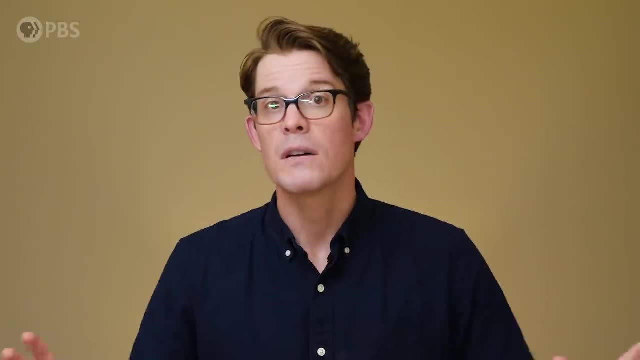 radiation escaped into the air because of a meltdown. Finally, in Fukushima, Japan, a meltdown contaminated the area, but was contained enough to minimize the human health effects. All these meltdowns are being studied today, so we can better understand the effects of radiation on humans and the environment. These accidents, while they're pretty scary, are rare. A more pressing concern is what to do with spent nuclear fuel. Uranium stays radioactive for a very, very, very long time, so used fuel rods must be stored safely somewhere for a very, very, very long time. 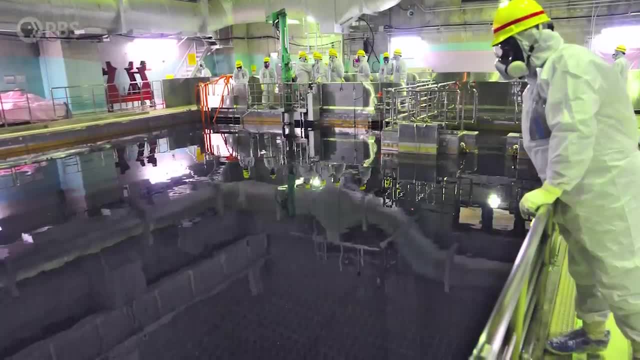 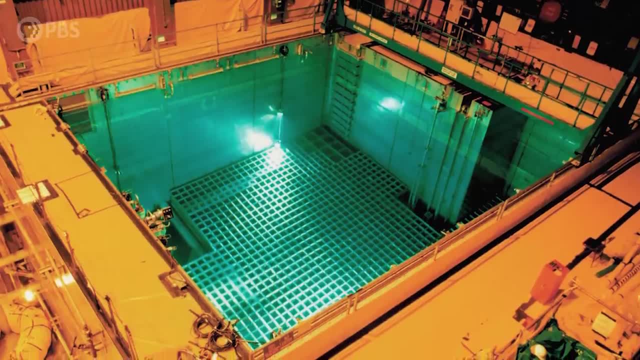 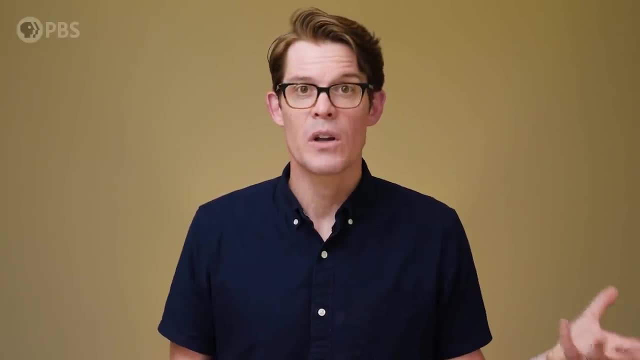 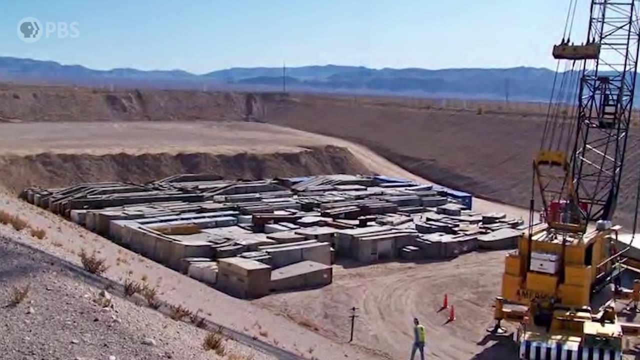 Currently, most is stored temporarily on-site at nuclear power plants, in large pools of water in specialized buildings. How to permanently handle such waste is a very real concern when it comes to generating energy from nuclear fission, Especially because countries like the United States and Australia have a bad habit of dumping. 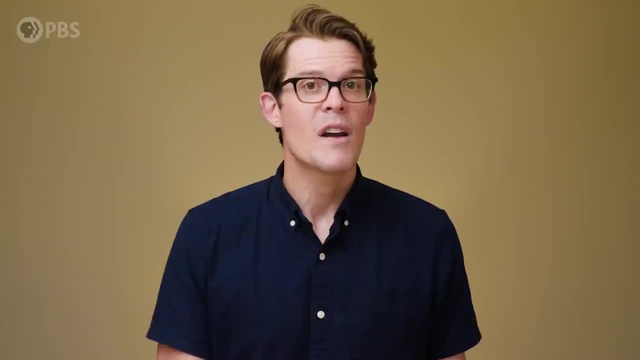 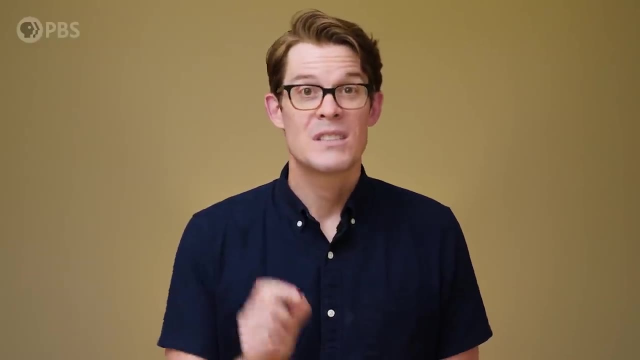 this waste on indigenous land. So while there are very real environmental benefits to using nuclear energy- not many emissions- there are potentially negative consequences, particularly in the context of environmental justice. Now we've covered all the major non-renewable forms of energy generation. Basically for coal, gas and uranium. we consume these resources at a rate that's way higher than they can be naturally replenished. While it may take millions of years for coal to form, we can mine it and burn it within days. This type of energy use is unthinkable. 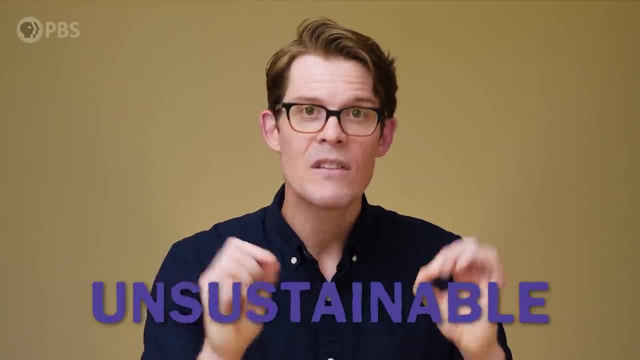 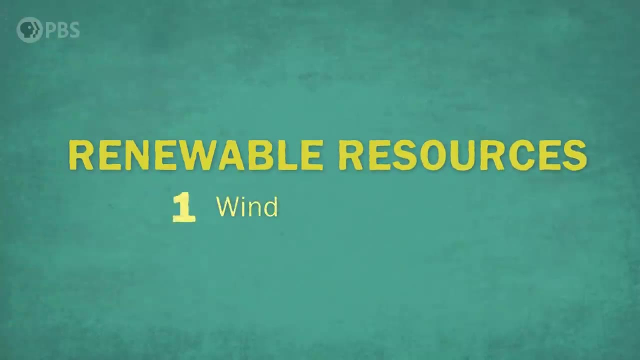 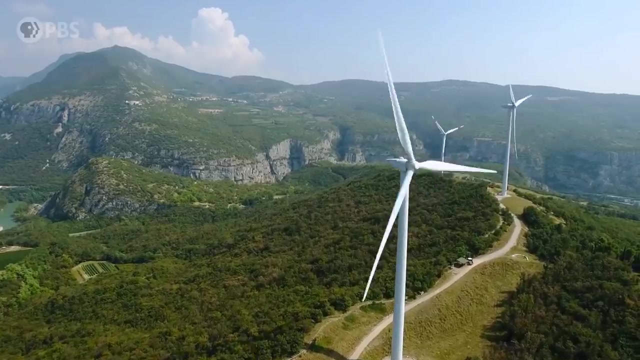 And, as we've talked about, it can have intense environmental impacts. But, shocker, there are ways to generate energy using renewable resources like wind, water, the heat in the earth and sunlight, With wind energy. wind spins a turbine, a very big turbine which rotates, a generator. 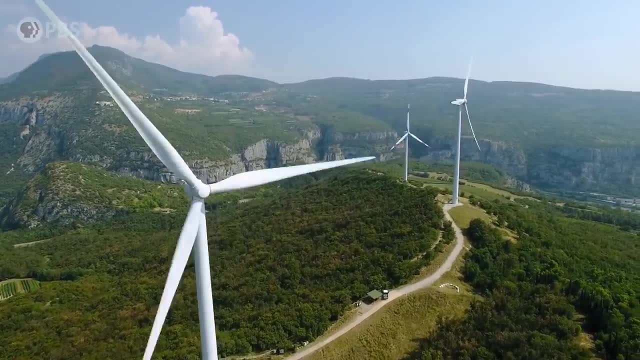 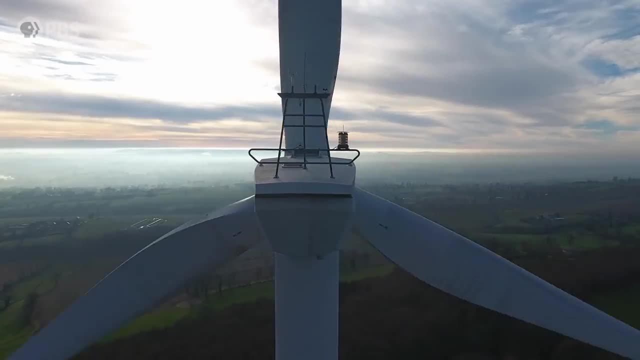 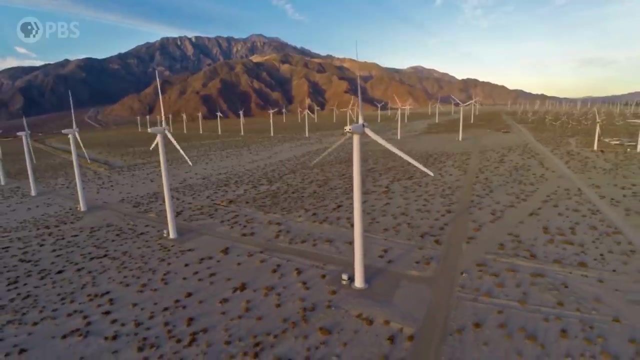 to produce energy. Thanks to the sun and earth's rotation, wind is renewable. We aren't running out of it ever And, aside from the initial production and construction of a wind turbine, no emissions are produced directly from it. Wind turbines, as beautiful as they are, are not without their drawbacks. 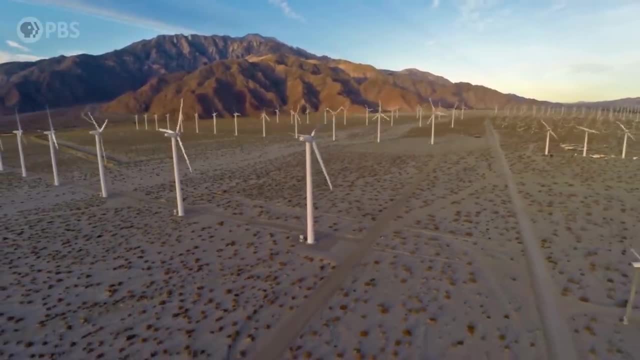 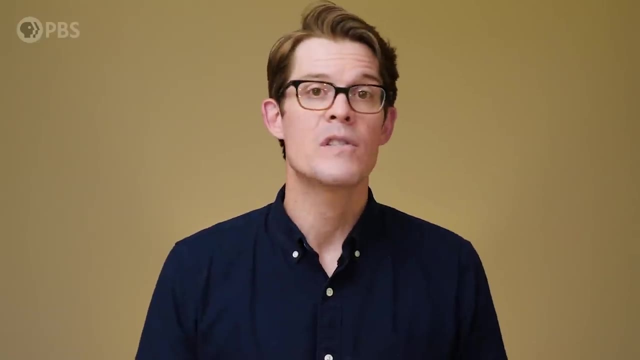 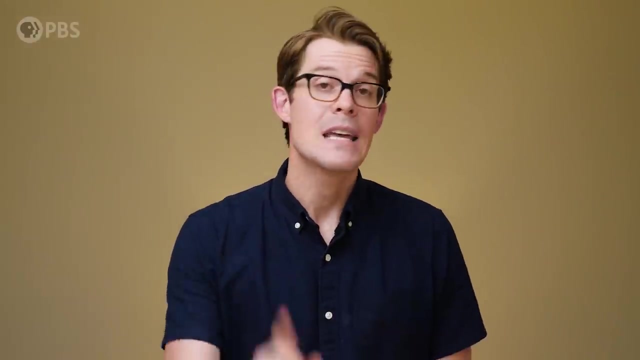 From an ecological perspective. the turbines do pose a risk to birds and bats. The construction of a field of wind turbines does result in some habitat loss. This can be mitigated somewhat with careful site selection and is just one of many ways that environmental scientists can be involved with energy production. And it is worth noting that the emissions from extracting and burning non-renewable sources like coal and gas do a lot more damage to the environment than they do to the environment. The main drawbacks of wind energy are location- not everywhere has wind- and intermittency. Places that are windy aren't windy all the time. Without careful planning, the electricity production of a wind turbine may not match the demand of the consumers. Intermittency is the biggest hurdle for energy generation, like wind and solar, But well-designed and managed grids with additional forms of energy storage can solve this problem. 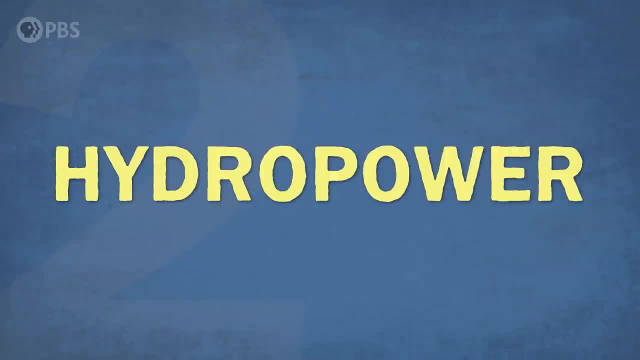 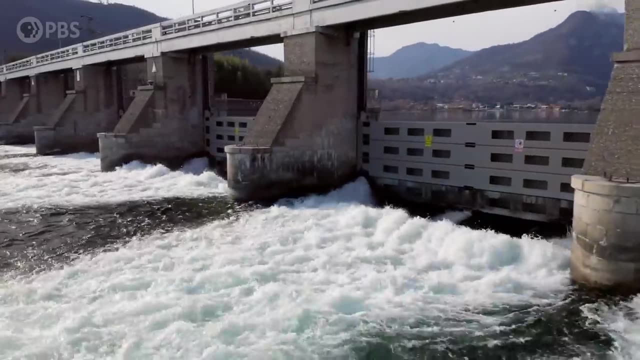 OK, Let's get started. OK, On to hydropower. Instead of using the motion of wind, a hydroelectric dam uses the motion of flowing water to generate energy. A dam controls the flow of water in a river, then creates a reservoir. 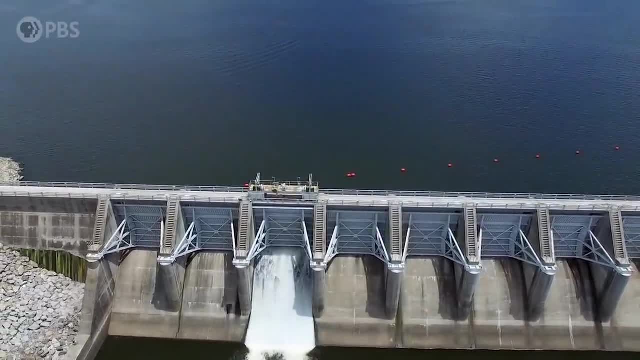 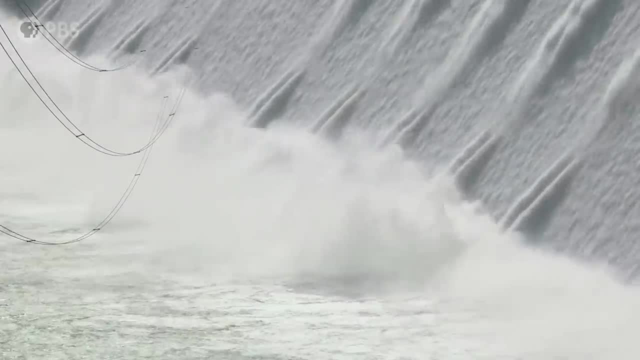 The water held in this reservoir has potential energy and the more water and the larger the difference in height between the reservoir and water downstream, the more potential energy. When that water is released and channeled through the dam, that potential energy is converted to kinetic energy and can spin the turbine and generator. 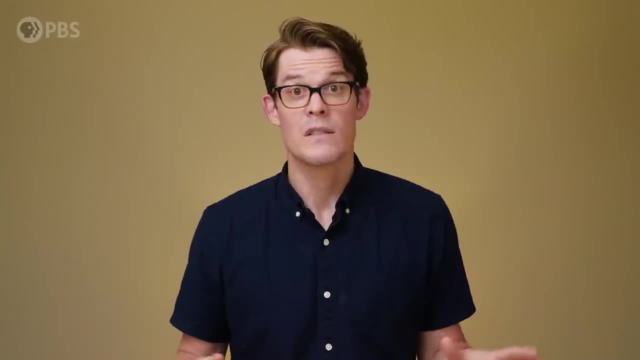 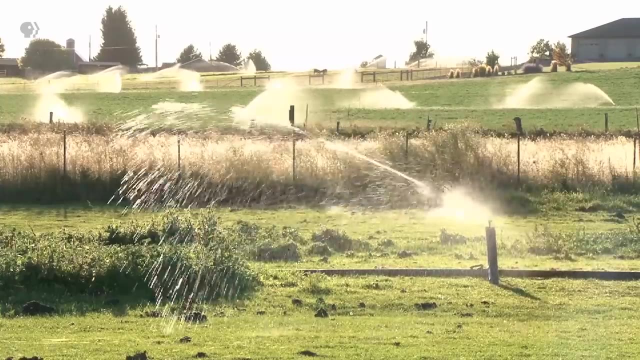 People have been producing energy this way for a really long time and dams do have a lot of benefits. That reservoir can be used for recreational activities, commercial fishing or agricultural irrigation. But dams are highly location-specific, need the right amount of water and topography. 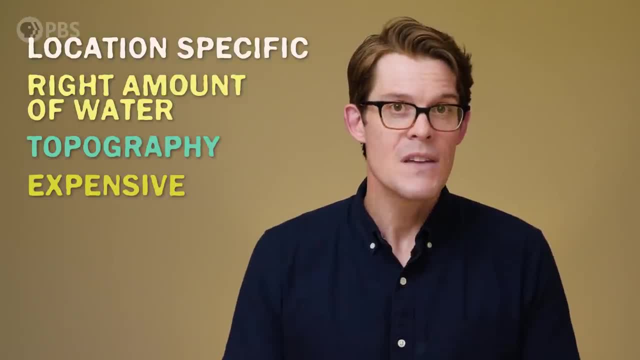 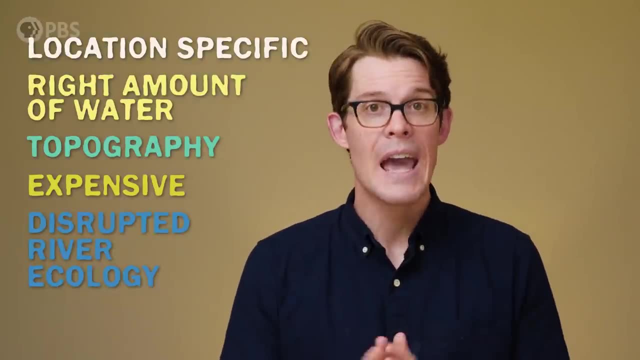 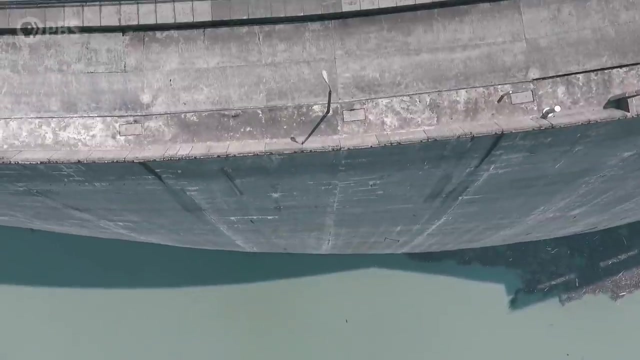 and constructing a dam is super expensive. Plus, there is a significant disruption of the river ecology And, while long considered an emissions-free source of energy, hydroelectric dams can have a lot of emissions. Not only is the construction expensive, The construction is extremely carbon-emitting because of the sheer amount of concrete used. 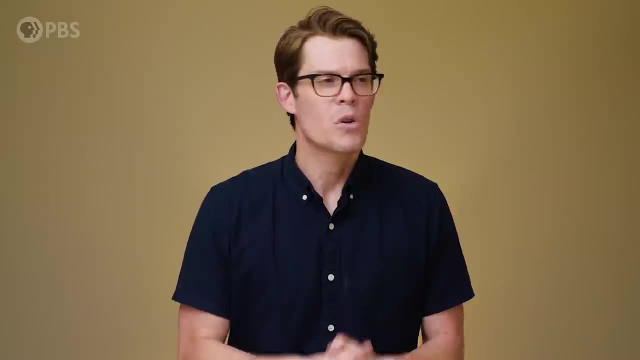 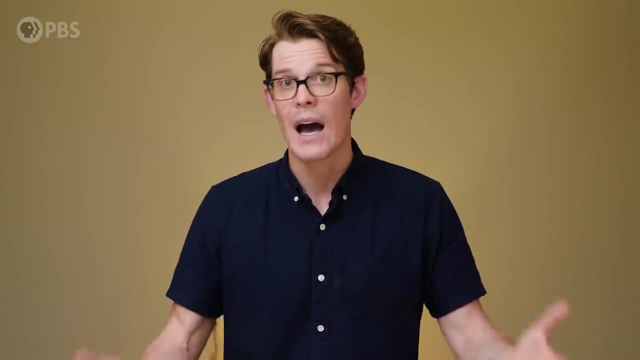 in building a hydroelectric dam But also creating that reservoir. it ends up flooding a lot of land. That organic material previously on the land can't survive under water. it dies and starts to decompose, And that decomposition releases greenhouse gases. This can be mitigated, and there are hydroelectric dams with reservoirs that serve as carbon sinks. This means that more life grows in them that draws down carbon than decomposes into the river. This needs to be taken into account when the dam and reservoir are constructed. 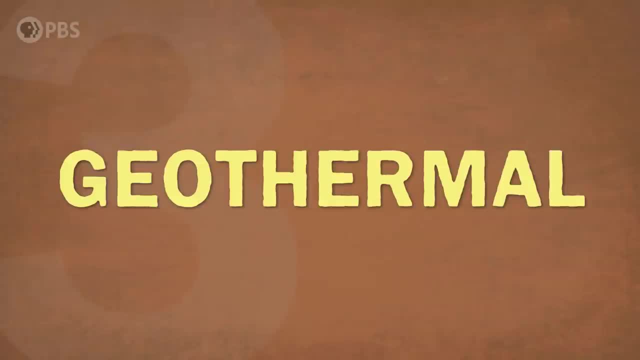 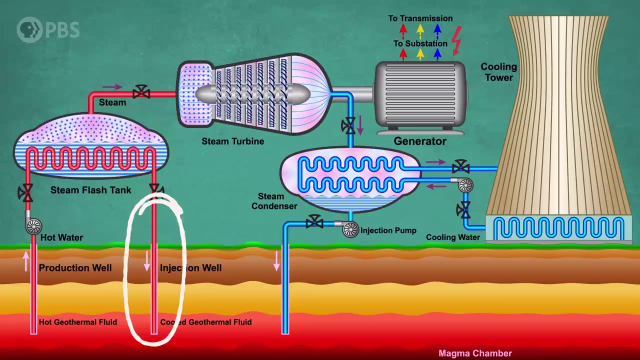 And now for our last turbine and generator energy source: geothermal. Geothermal uses the heat from deep within the earth to generate steam to spin the turbine and generator. Water or another liquid travels deep underground, is heated and then heads back to the surface. 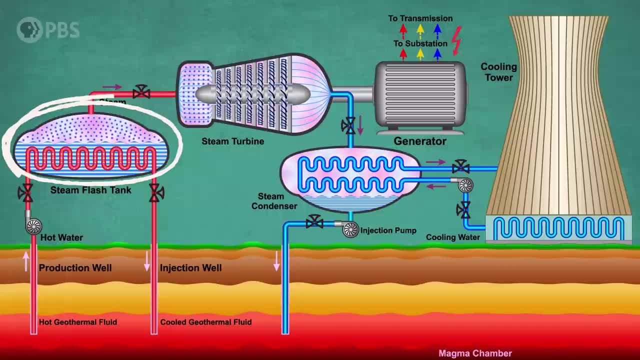 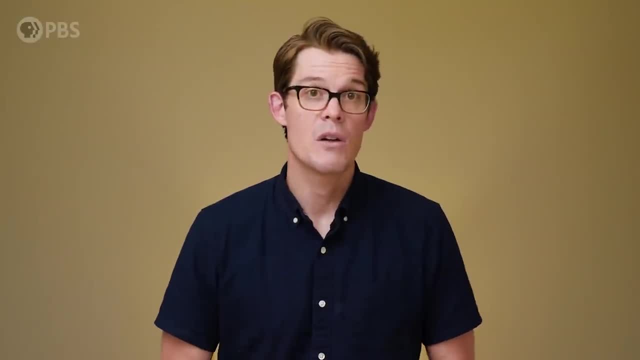 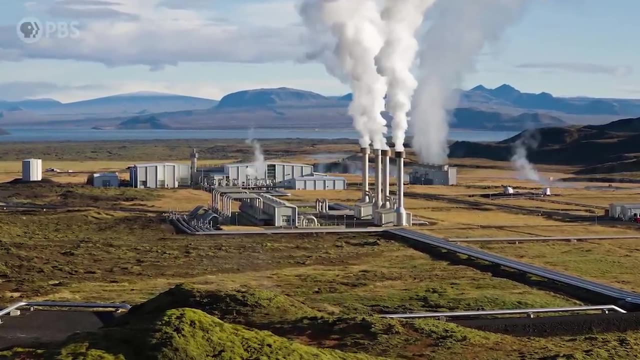 where it's pressurized, heating it up further, releasing steam to turn the turbine, and then the now-cooled water heads back underground to do it all over again. The process of geothermal energy generation doesn't release emissions or pollutants, with the exception of the initial construction and the accidental release of hydrogen sulfide. 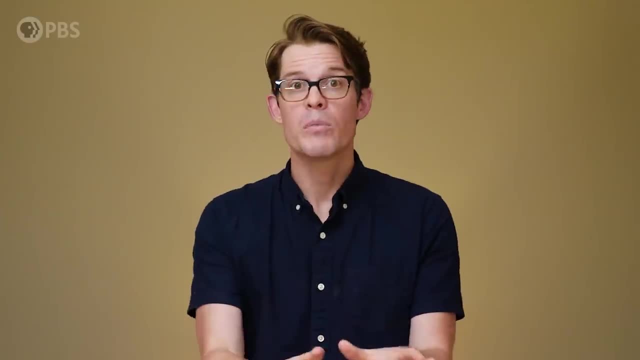 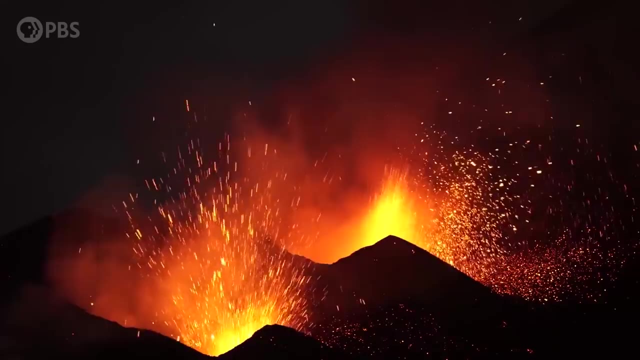 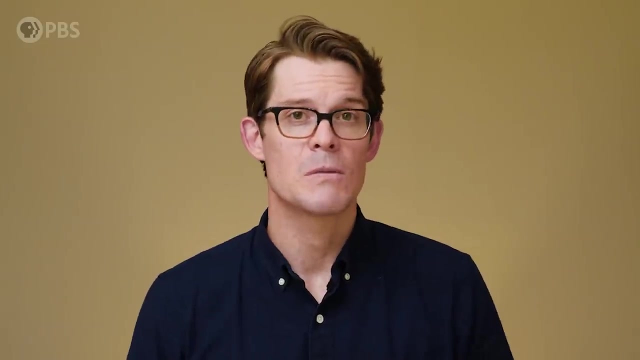 from groundwater into the atmosphere. However, geothermal plants work where the heat from the earth's inner layers are close to the surface, which limits it to areas with lots of volcanic activity or near the edges of tectonic plates, And a lot of the best locations for geothermal are already in use. 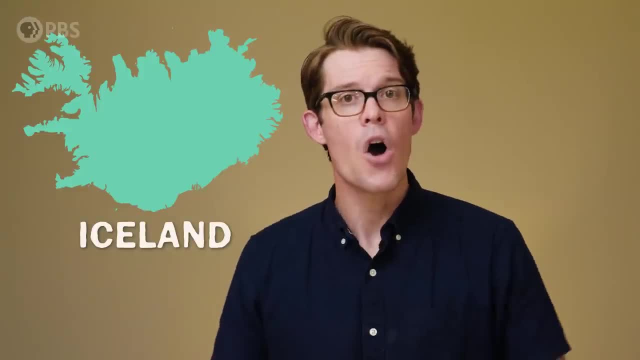 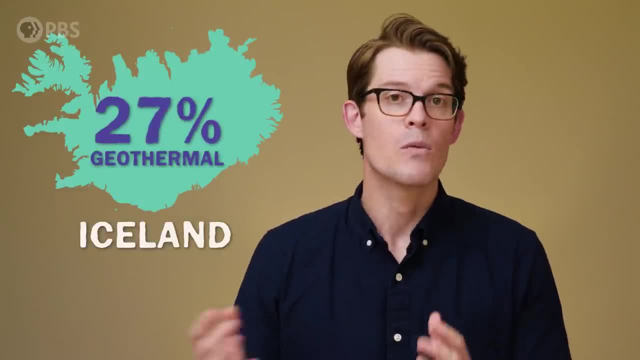 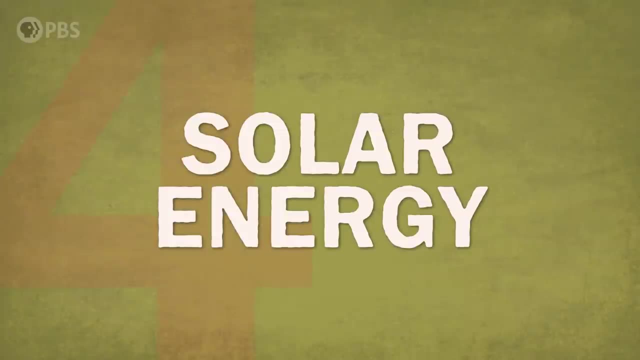 In 2016,. about 27% from geothermal and the rest from hydropower. And last but certainly not least, we have solar energy. Solar energy production, unlike everything else we've talked about, doesn't use an electromagnetic generator. Instead, when light hits, the semiconductors. 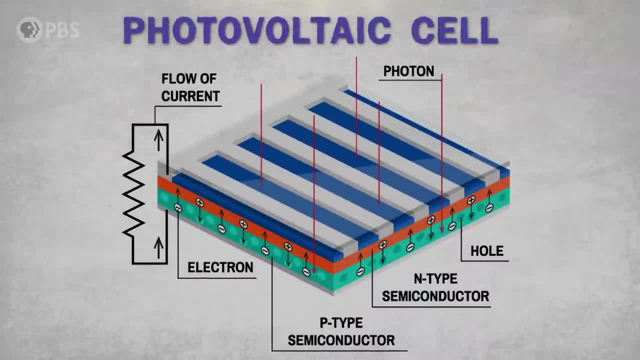 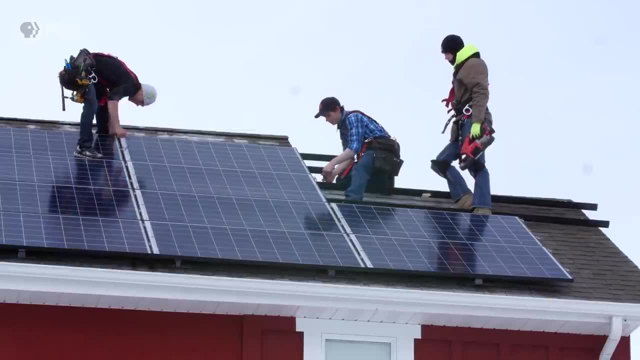 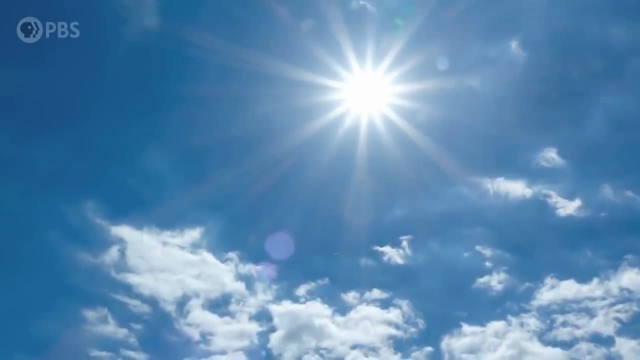 within the photovoltaic cells. the photons in the sun's energy knock electrons free and form an electron flow. Solar panels have way fewer moving parts and are much easier and cheaper to construct than any of the other forms of energy generation we've talked about. Plus, their only location dependency is that they need to see the sun, Sure some places. like a desert in the US Southwest will be more efficient than the cloudy forests of British Columbia, but solar panels will produce at least some energy in any place that the sun hits. Solar panels have gotten increasingly less expensive in the last few years In many places. solar energy generation is cheaper than coal and gas, and it looks like it'll only get cheaper in the future. But like wind, the sun is an intermittent energy source. Solar panels won't generate energy at night, And while energy generation from solar doesn't release any emissions, solar panels do rely on really specific materials to function. 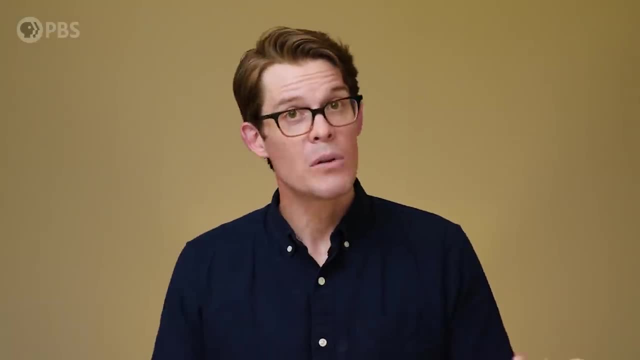 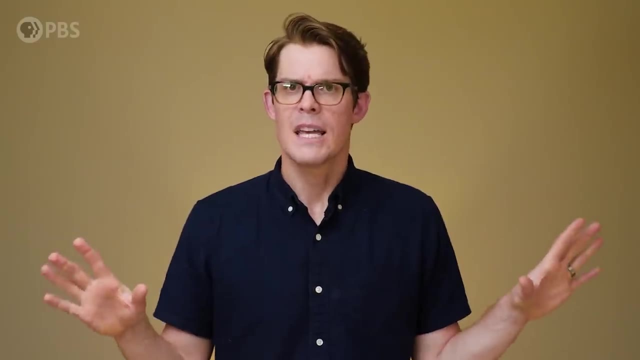 and many of those need to be mined, which can create emissions and pollution all on its own, And those mines are often very dangerous for the people working in them. Okay, let's take a minute to catch our breath, because covering all that energy, 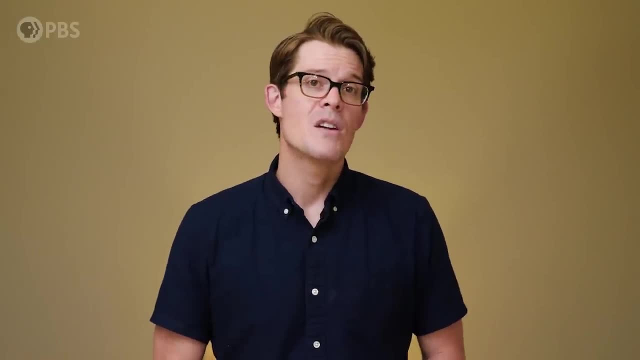 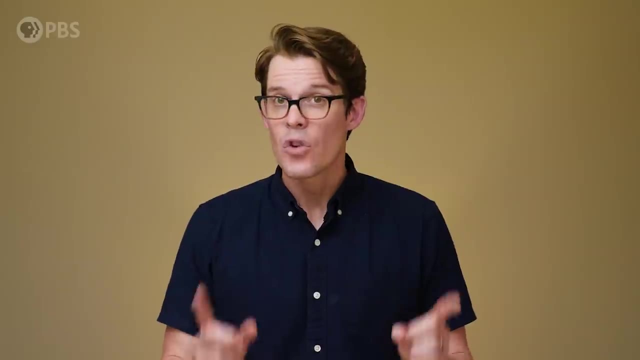 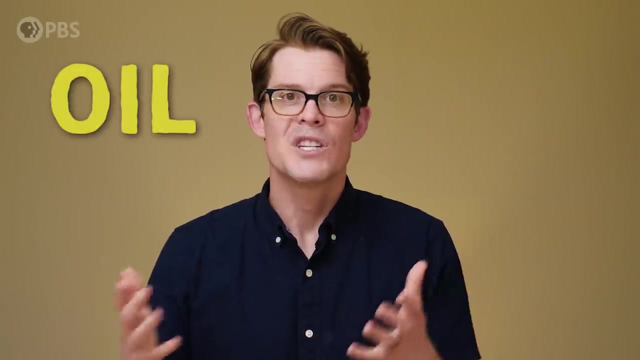 took a lot of energy. Depending on where you live, the percentage of energy from each of these sources can be pretty different And it's changing year to year as renewable sources get cheaper and the global demand to reduce greenhouse gases rises. But we've got one last fossil fuel to talk about, oil. We generally don't use oil to generate. 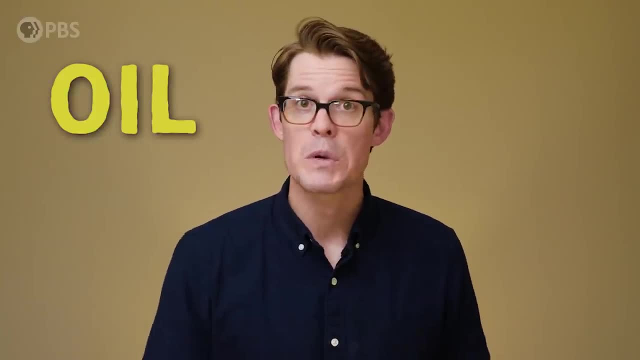 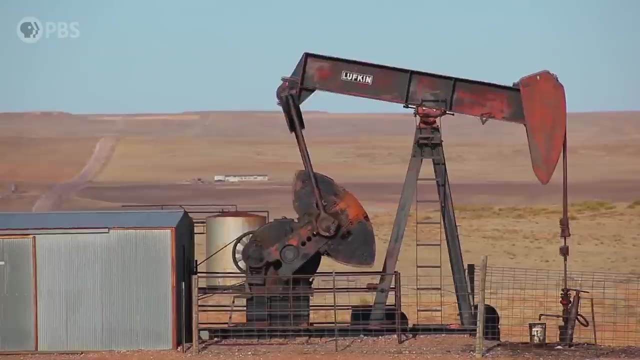 electrical energy. these days, rather, it's primarily used as a transportation fuel and to make plastics, while it is, in fact, a fuel that bears knowledge of the dirigibles of the second world. Oil, like fossil gas, is found in underground pockets, trapped in rock and accessible by 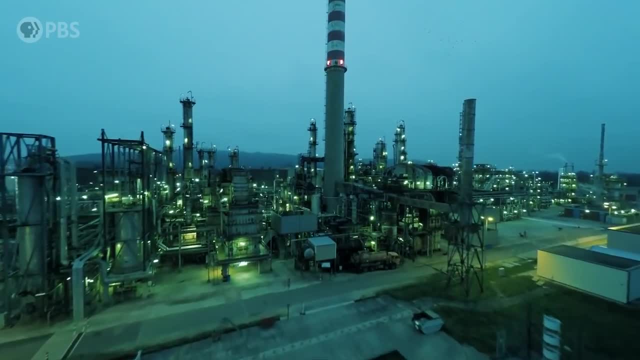 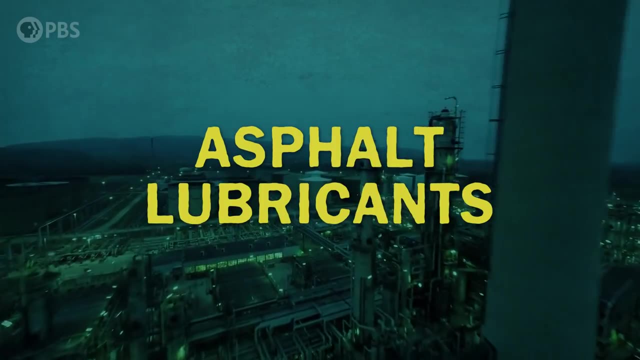 drilling. Once this crude petroleum is pumped from the ground, it's sent to a refinery, where it's separated out into different fuels, such as gasoline, diesel or aviation fuel, as well as products like asphalt and lubricants And- surprising no one- like the other fossil fuels. 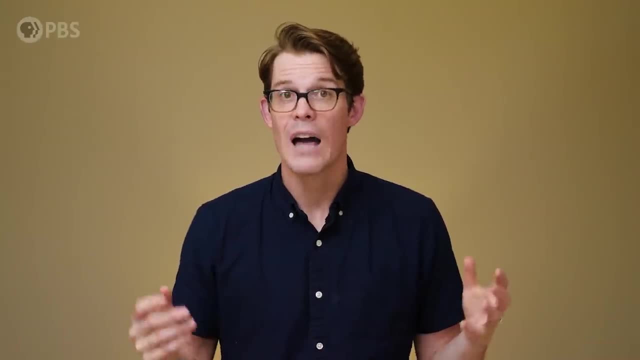 the combustion of oil results in air pollution and carbon dioxide emissions. And it's a lot of emissions Because, at least right now, nearly every car and train and bus, bus and car engine isviable, And it's a lot of emissions. 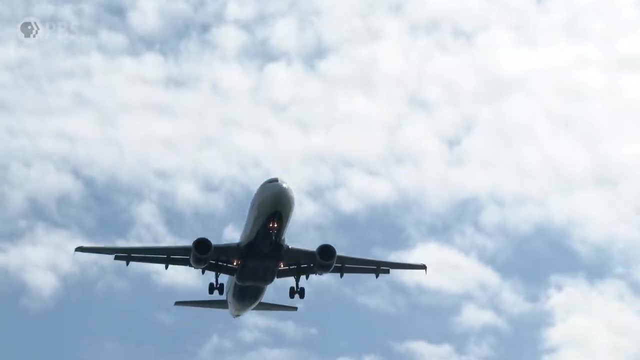 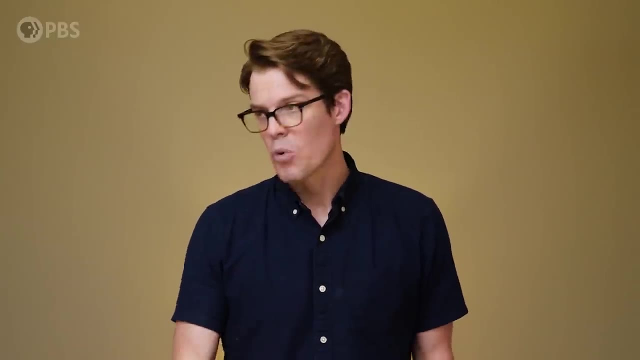 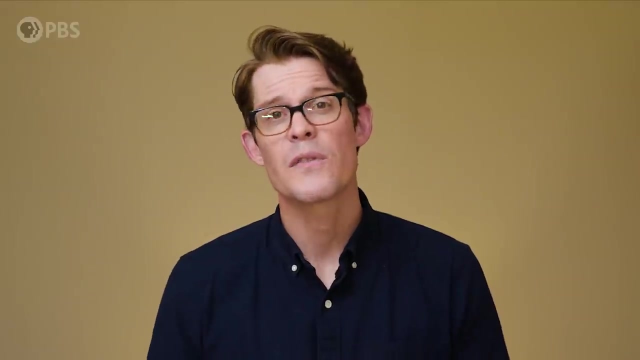 Right now, nearly every car and train and plane that you've ever seen, and the millions that you haven't, run on some form of oil pumping out carbon dioxide for every mile Or kilometer, depending on where you're from. One of the unique and deeply unfortunate environmental consequences of our use of oil is the frequency. 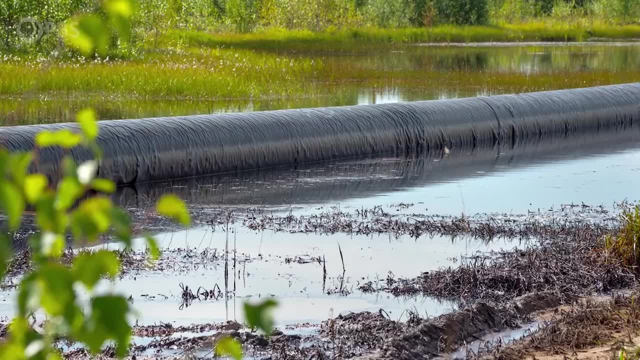 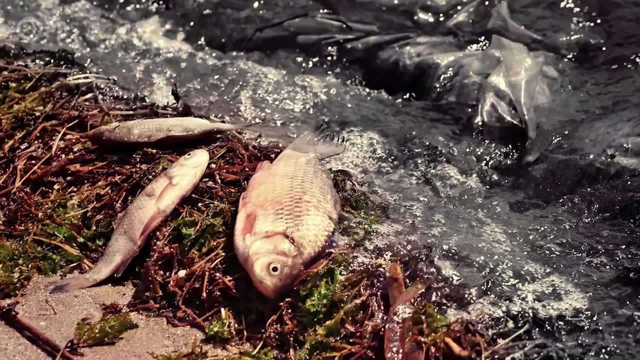 of oil spills during transport. Whether it's a pipeline leak or an oil spill from a tanker in the ocean, oil can cause lots of damage to both terrestrial and aquatic habitats. The largest oil spill in the US was in 2010, when BP's Deepwater Horizon exploded in. 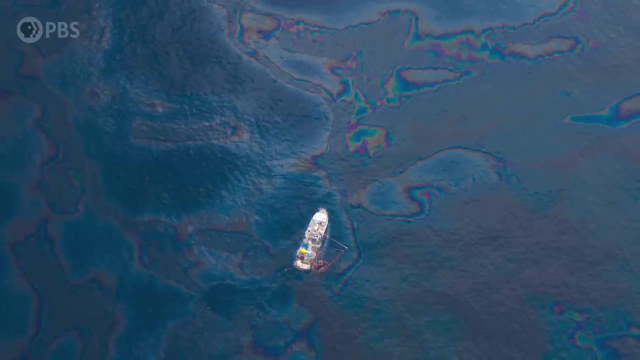 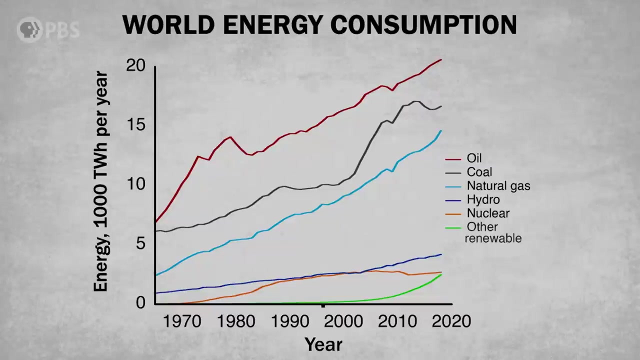 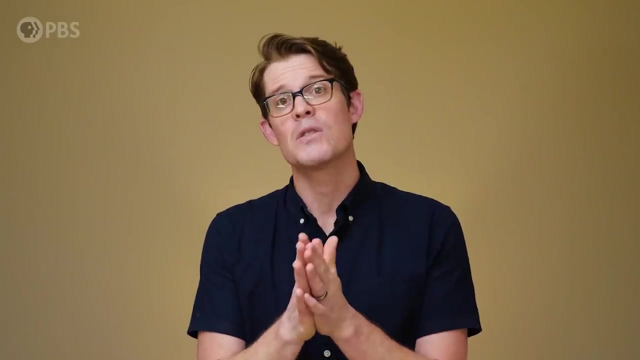 the Gulf of Mexico, resulting in millions of gallons of oil contaminating coastal and marine ecosystems. Now, if we look at global primary energy production, fossil fuels have and continue to dominate, despite the abundance of far more sustainable energy production options. But changing that is going to require massive global buy-in and a reframing of what energy